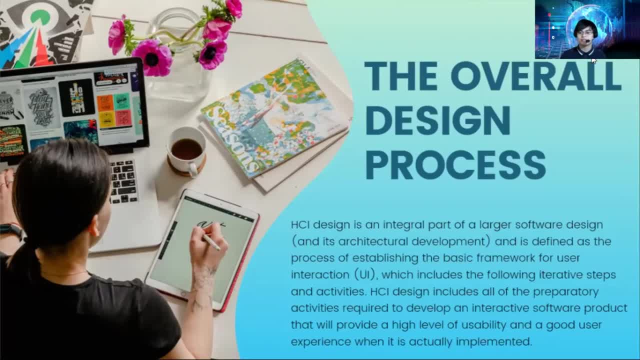 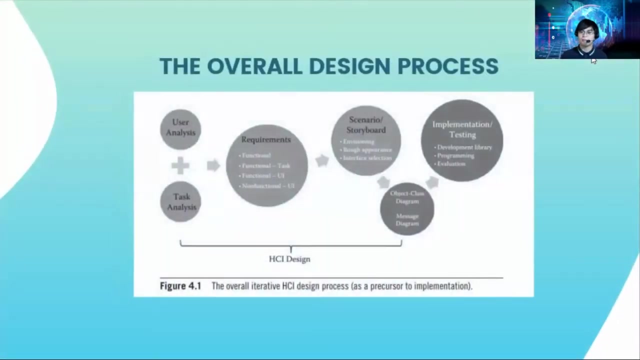 includes the following iterative steps and activities. So HCI design includes all the processes required to develop an interactive software product that will provide a high level of usability and a good user experience when it is actually implemented. So this is the very first step and it's very important. So we will be discussing this process. So, as you can see in 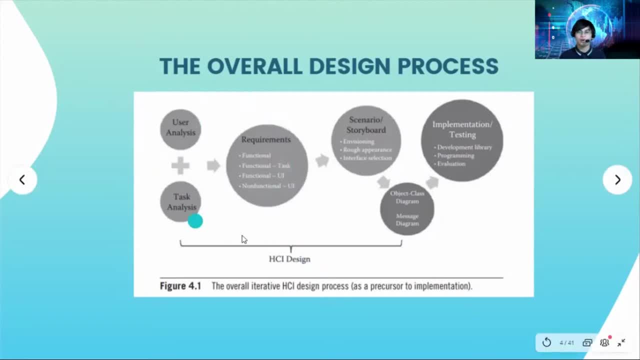 the in this image. this is the overall HCI design. So these are the different processes before it is being passed through the implementation or the testing phase. So for this course we will only be dealing this phase. So don't worry, because we're going to discuss that one by one. What is the user? 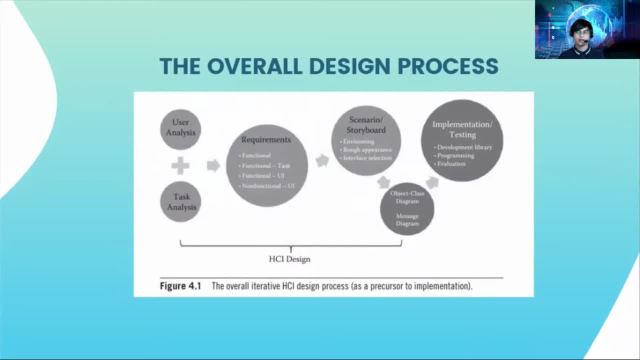 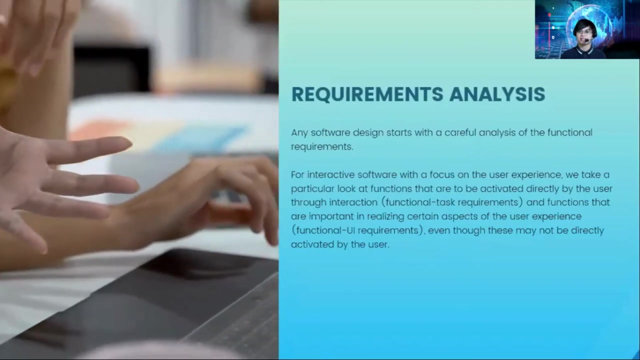 analysis, the task analysis, requirements, etc. Okay so this is the first step and this is the next step in the process. Okay so this is the look. This is the overall iterative HCI design process as a precursor to implementation. Okay so let's start with our first process. The first process is requirements analysis, or simply as 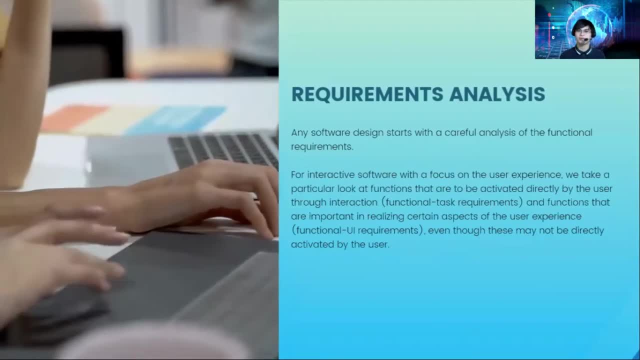 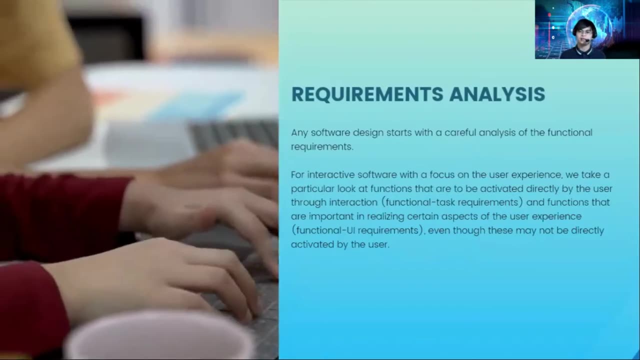 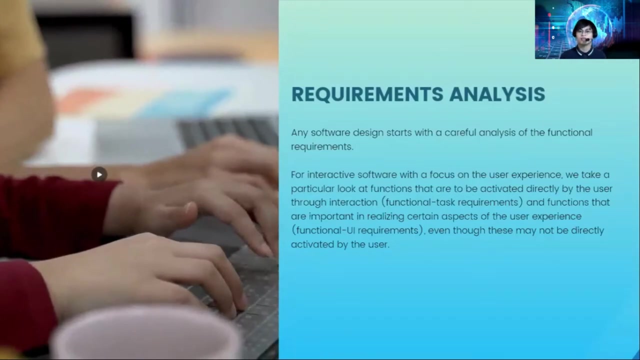 data gathering. When you actually design something or research, you gather data. So any software design starts with a careful analysis of the functional requirements. Okay so for interactive software with a focus on the user experience, we take a particular look at the functions that be activated directly by the user through interaction. So this is also called 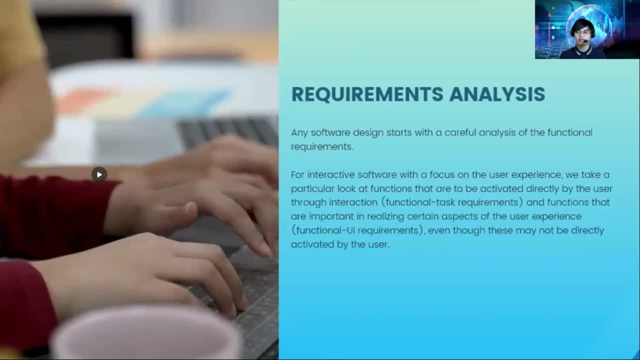 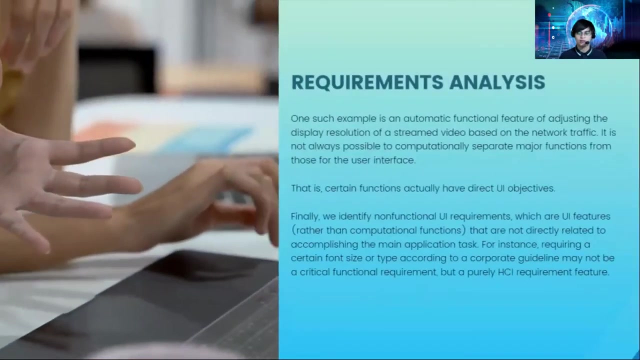 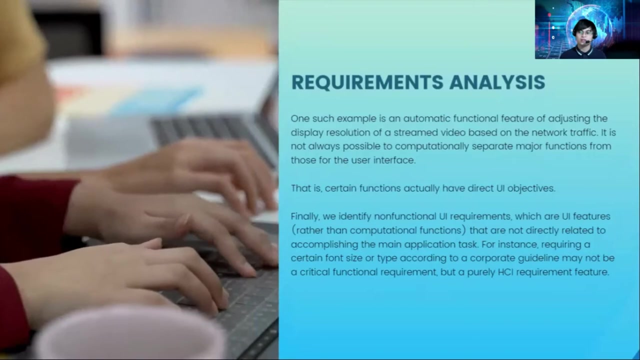 the functional task requirements And functions that are important in realizing certain aspects of the user experience or the functional requirements, even though this may not be directly activated by the user. So let's discuss further. One such example is an automatic functional feature of adjusting the display resolution of a streamed 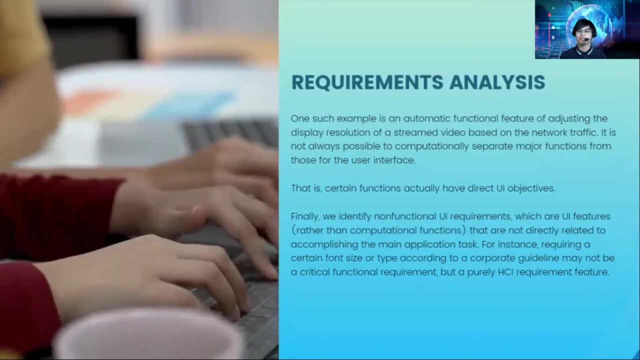 video based on the network traffic. So it is not always possible to computationally separate major from those or for the user interface, That is, certain functions actually have direct UI objectives. So, finally, we identify non-functional UI requirements, which are UI features rather than. 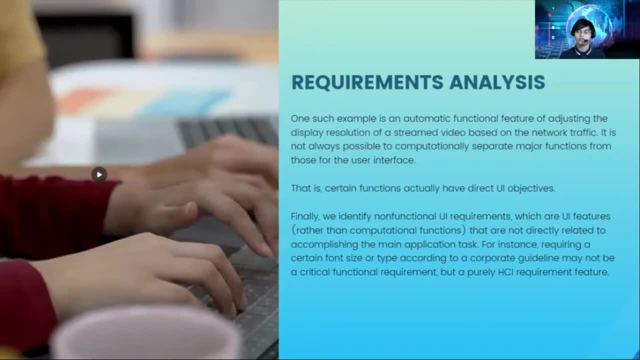 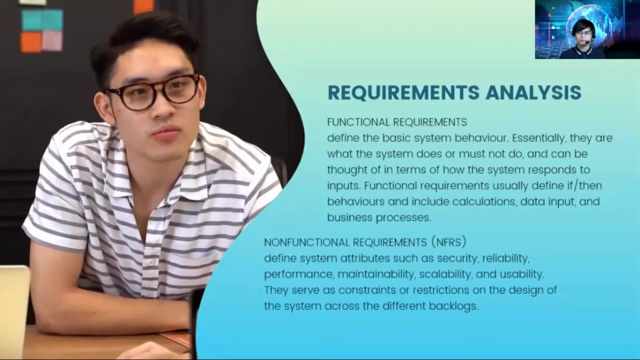 computational functions that are not directly related to accomplishing the main application tasks. So, for instance, requiring a certain function to be executed using a system behavior. it may be a function of a specific type or a type according to a corporate guideline, but a purely a UI requirement feature. So let's discuss further and let me give you an example. 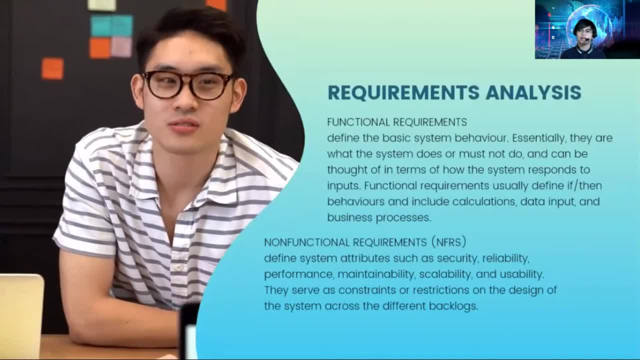 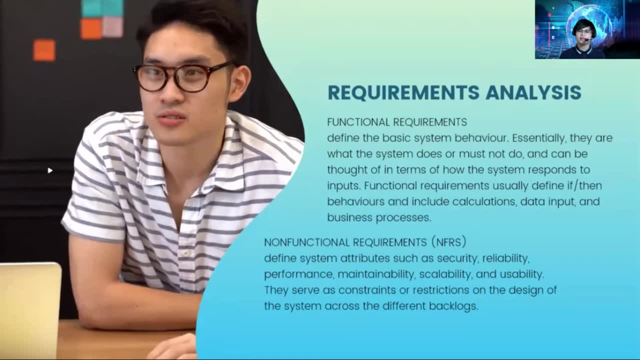 Okay. so in requirements analysis, guys, you must know the functional and the non-functional requirements. So what are these functional requirements? These are defined as the basic system behavior. essentially, they are what the system does or must not do. okay and can be thought in. 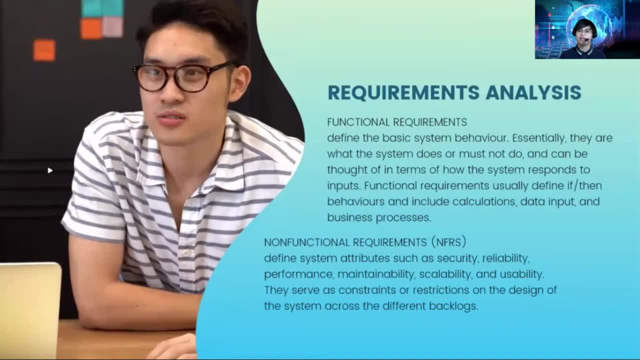 thought of in terms of how the system responds to inputs. so functional requirements usually define, if then behaviors and include calculations, data input and business processes. functional requirements, guys, is as easy as the features of your system. what are the different features of your software or your system name? give what, let us say, for example, um, an application where it will. 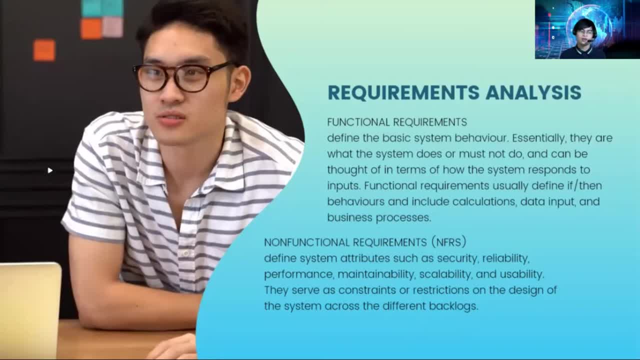 detect a, a user, who, if a user is wearing or not wearing a mask, so something in an application. so the functional requirements would that? be well, that application successfully detects the face of of a user. one young feature. okay, the non-functional requirements is this: is defined system attributes such as security, reliability, performance. 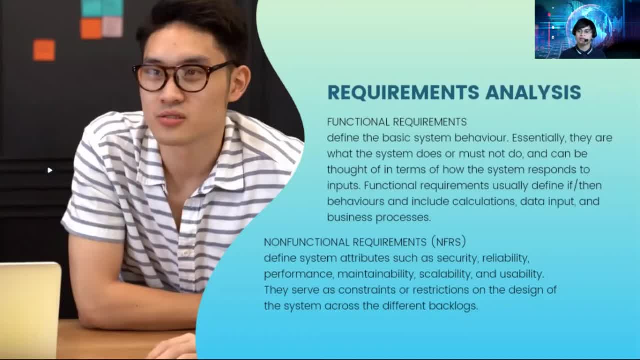 maintainability, scalability and usability. they serve as constraints or restrictions on the design of the system across the different backlogs. so the non-functional requirements is again um attribution shop, such as the security okay, reliability, performance, usability and etc. the function is the main features. i hope again, the functional is the main features. 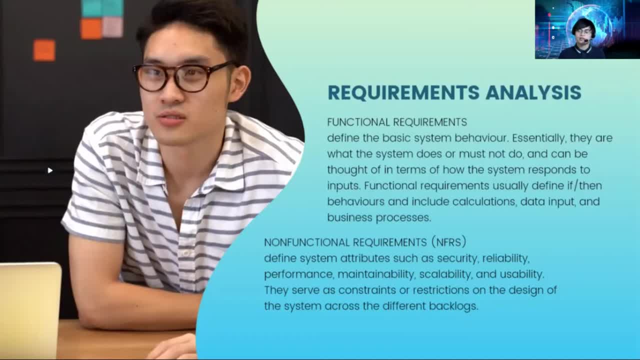 and the non-functional are the attributes of such as security, reliability, performance, maintainability and usability. okay, so, uh, those where cons are only more are, get on. how are you analyze the requirements? so it's very important. no, but you understand the functional and then the non-functional requirements, okay. 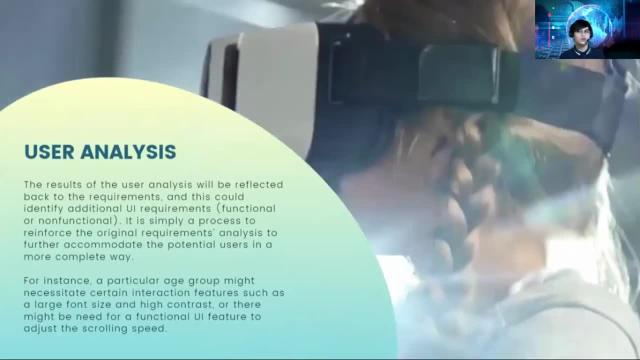 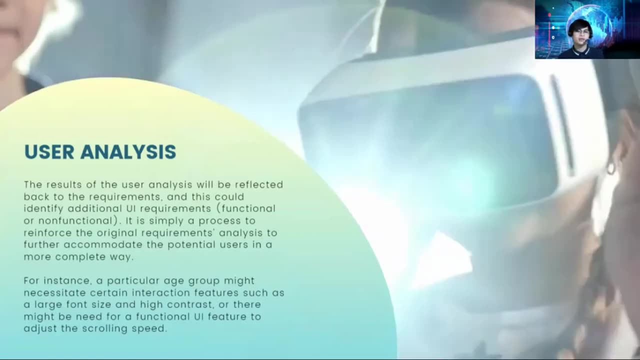 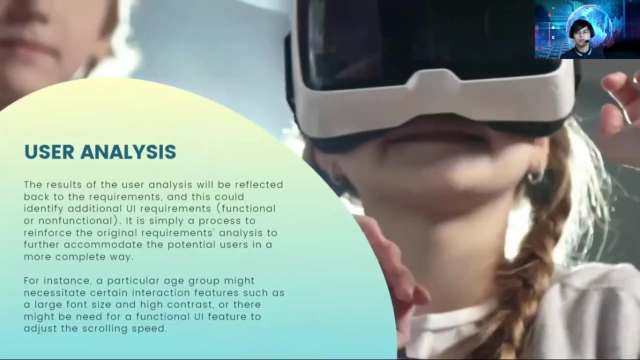 next step: okay, user analysis. you analyze again and then you need to know who will be using your software. so that's very important, but as someone almost software, okay, so in user analysis the results of the user analysis will be reflected back to the requirements and this could identify additional uai requirements. 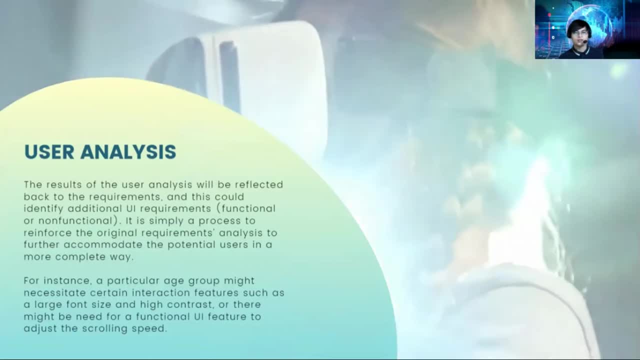 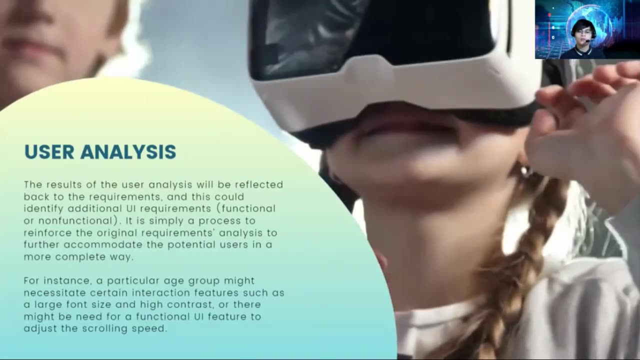 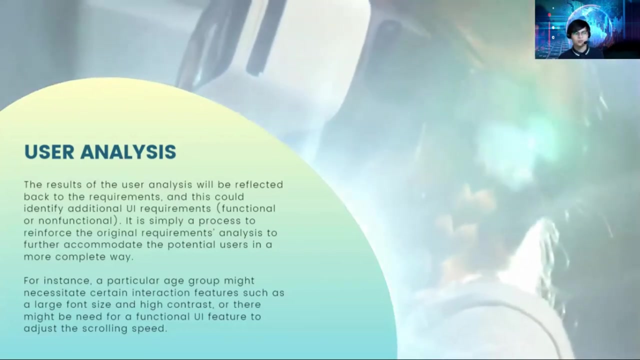 so functional or non-functional. so it is simply as the process to reinforce the original requirements analysis, to further accomplish the functional requirements of the software, so in the user analysis, further accommodate the potential users in a more complete way. So, for instance, a particular age group might necessitate certain interaction features such as a large font size and high. 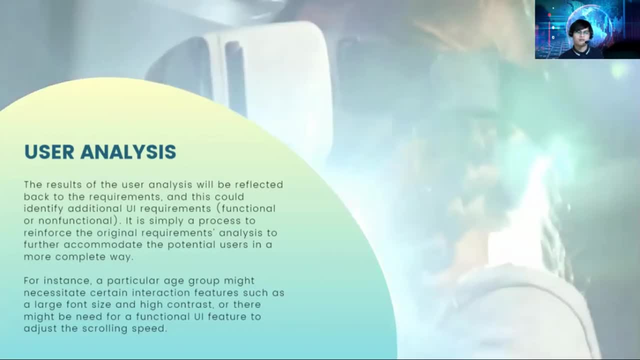 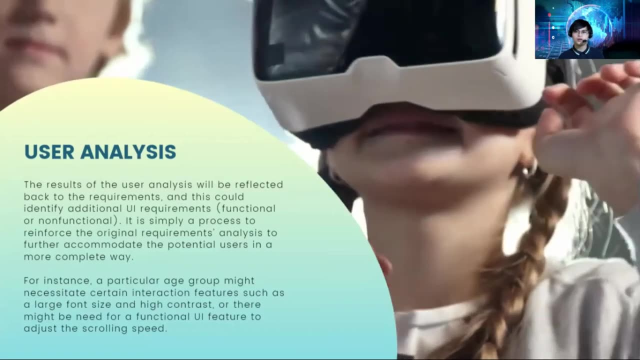 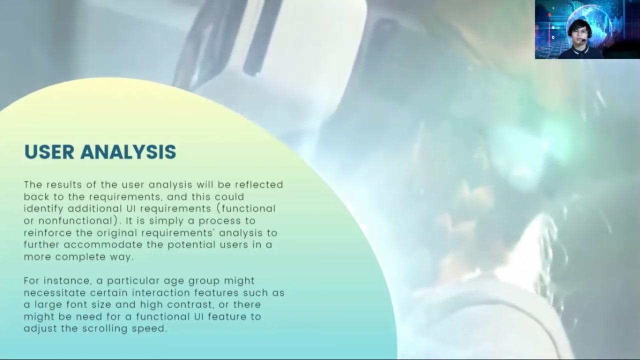 contrast, or there might be a need of functional UI features to adjust the scrolling speed or etc. Okay, so, for example, the user of your application will include the senior citizens or adults. They will learn how to use the software. So your application would be of: 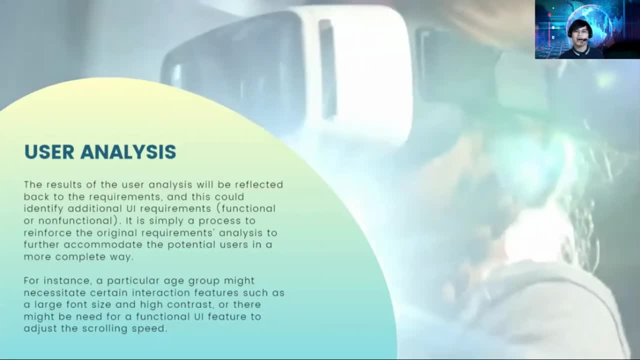 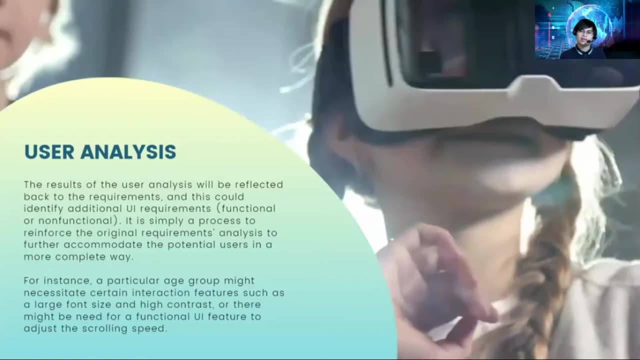 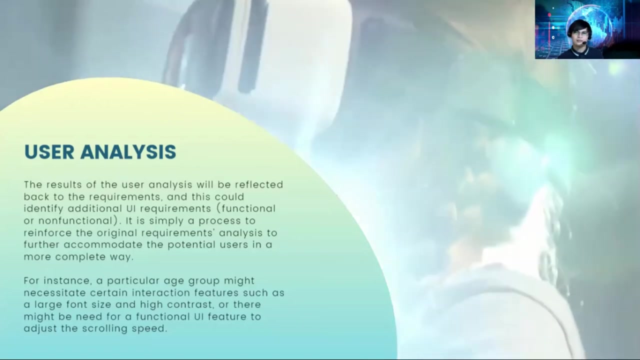 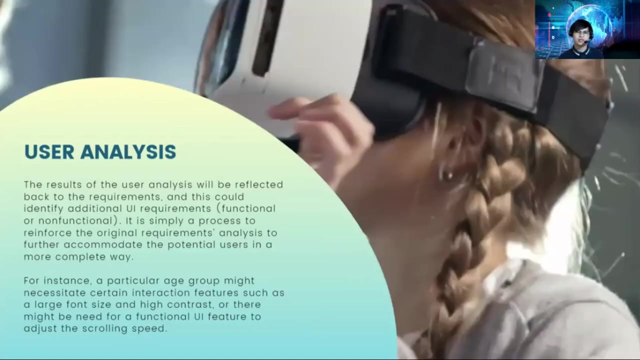 course, a large font size, high icons or something like that, And also if your application will be used by students or middle-aged adults. what are the other options in your system? Okay, Would it be features that the user will have an option to actually update? you know to. 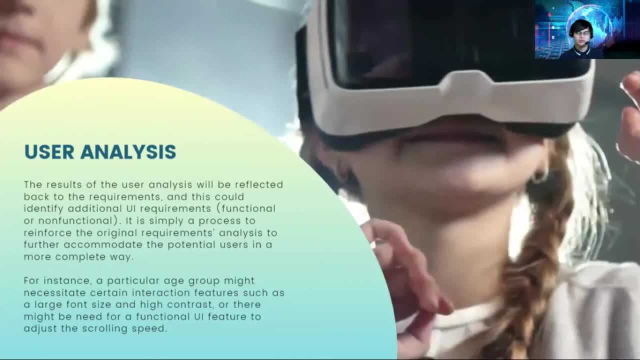 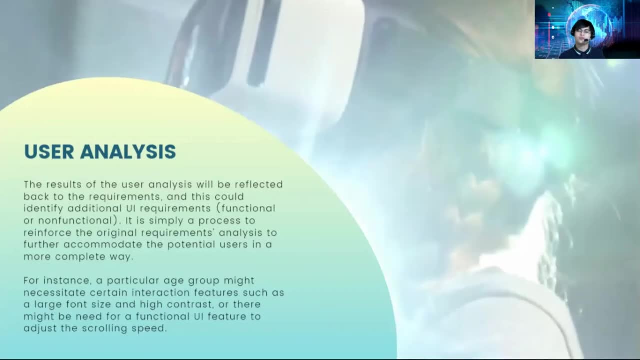 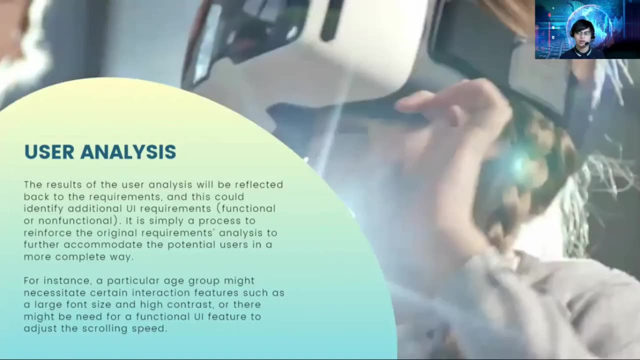 change the font size, the font color or etc. So it's very important that when you design a software, you analyze who will going to use your software. Okay, The user analysis phase, And I hope you guys have learned something. Okay, So that's it for our presentation. 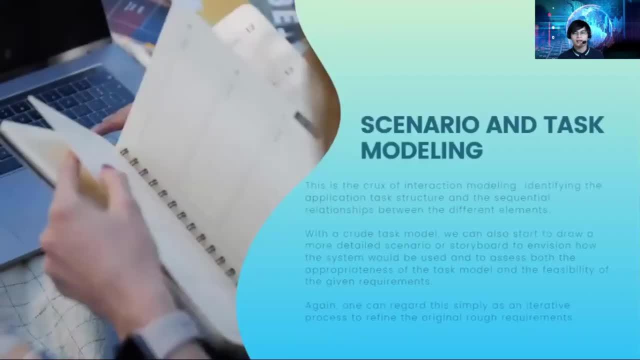 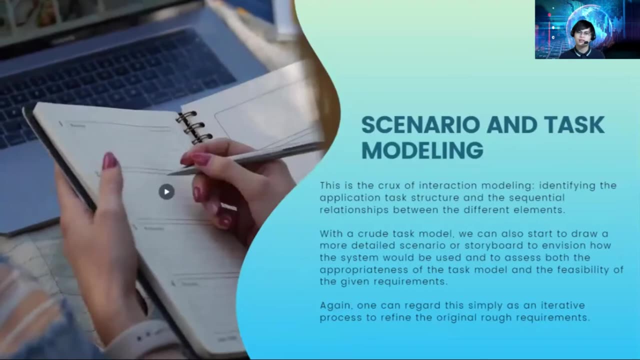 Next is the scenario and task modeling. Okay, of course, after gathering the requirements, getting what would be the different features, how we're going to use the applications, we're going to go with the scenario and then task modeling. What are the different jobs or tasks? 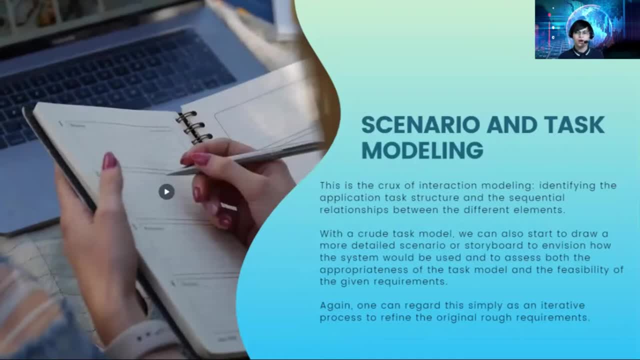 that your application is going to do Okay. so this is the crux of interaction modeling: Identifying the application's task structure and the sequential relationships between the different elements. So with a current task model, we can also start to draw a more detailed scenario or a storyboard of. 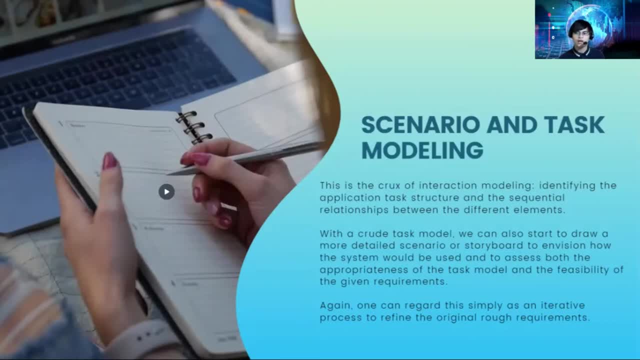 envision how the system will be used to assess both the appropriateness of the task model and the feasibility of the given requirements. So, again, one can regard this simply as an iterative process to refine the original rough requirements. okay, so you need to think of the different scenarios to what will gonna happen if my own embattled 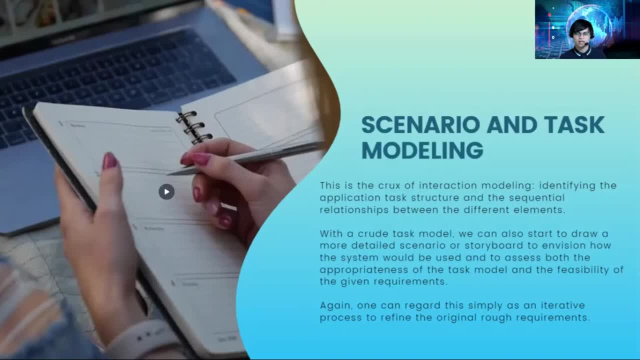 user. you define the task and up at my own, amahita boo say mo on application. okay, of course the developer will, but base Shasha Monica, bomb what name? on Mama task. I'm a different scenario. okay, so that's the scenario. don't worry, guess what will be? we have an example. no, we. 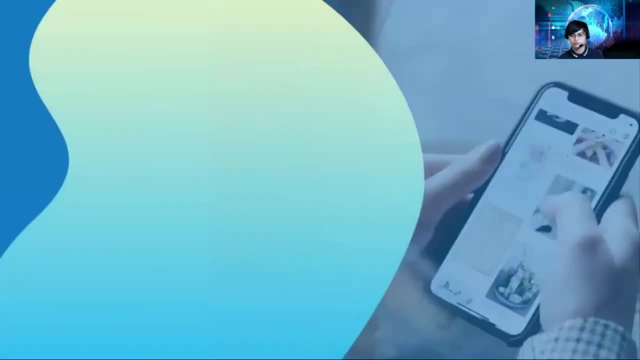 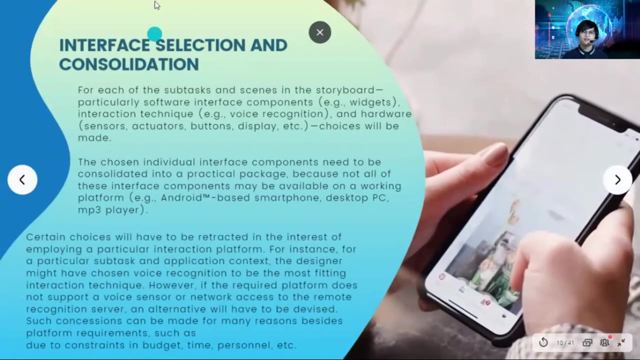 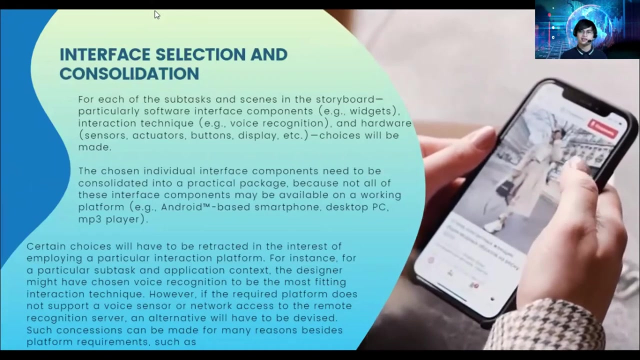 'll be giving an example for this. okay, so after that process, now I put die- we have interface selection and consolidation for each of the subtasks and since in the in the sub tasks, and since the task was created in the first sub tasks, and since in the the sub tasks were created in the 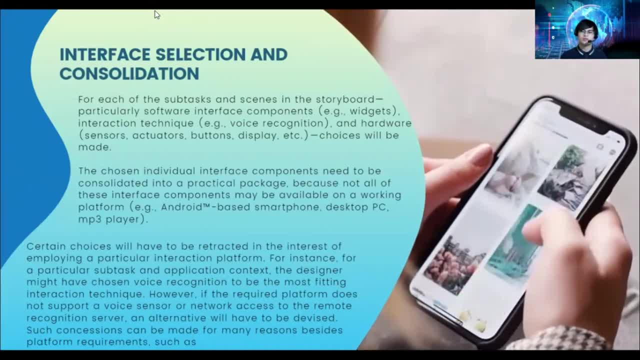 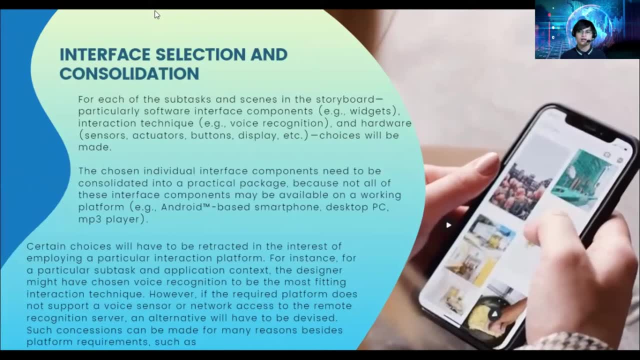 the storyboard, particularly software interface components: Example widgets, Interaction technique for the voice recognition and hardware sensors, actuators, buttons, display, etc. Choices will be made. The chosen individual interface components need to be consolidated into a practical package because not of all these interface components may be available on working. 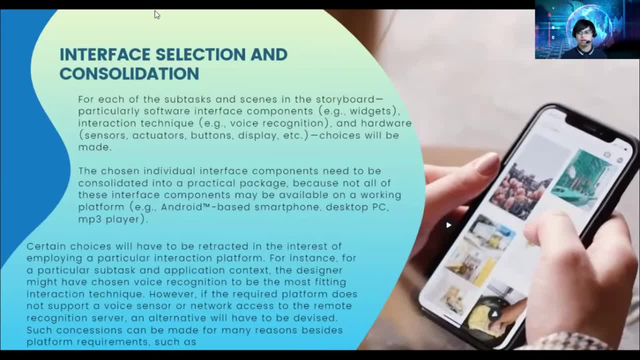 platform. that could either be in the Android, Android-based smartphones, desktop PC or mp3 player. Certain choices will have to be retracted in the interest of employing a particular interaction platform, For instance, for a particular subtask and application context the designer might have chosen. 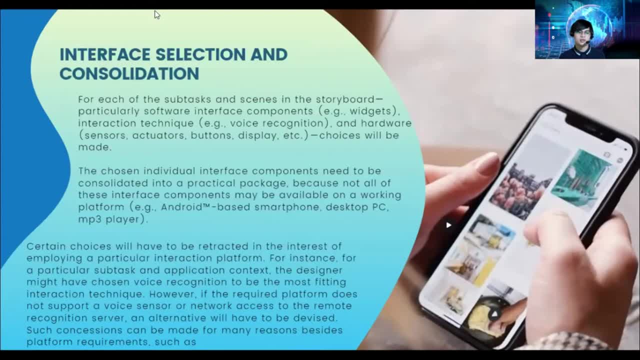 voice recognition Voice recognition to be the most fitting interaction technique. However, if the required platform does not support a voice sensor or network access to the remote recognition server, an alternative will have to be devised. So such conditions can be made for many reasons besides platform requirements. All such 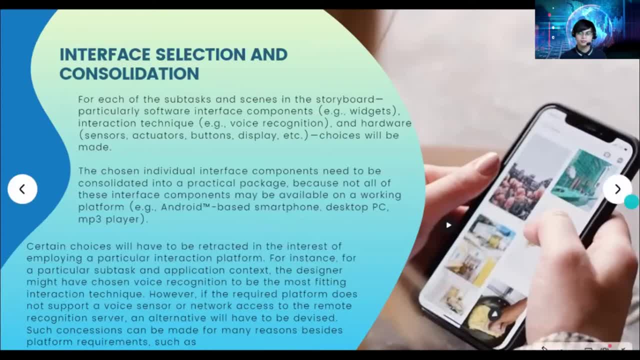 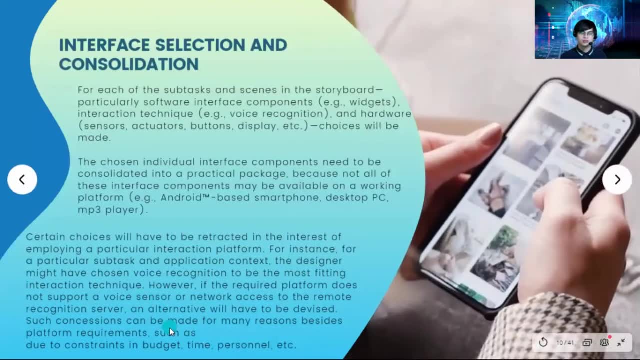 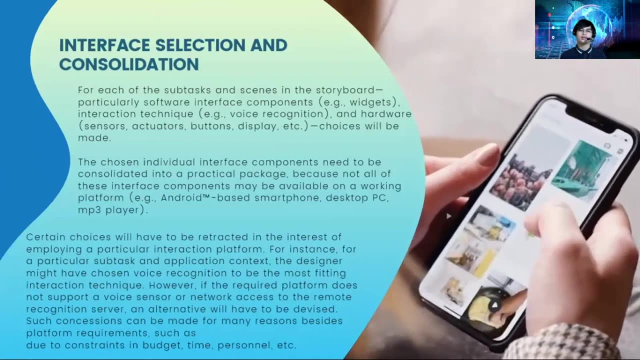 as such, as due to the constraints in budget, time and personnel. So it's very important that you should understand the interface, selection and consolidation. So again, for example, if an application is used, say sensor, you think how much He or She is aware of the? 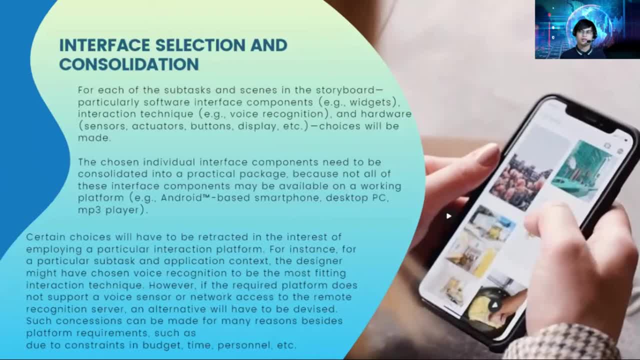 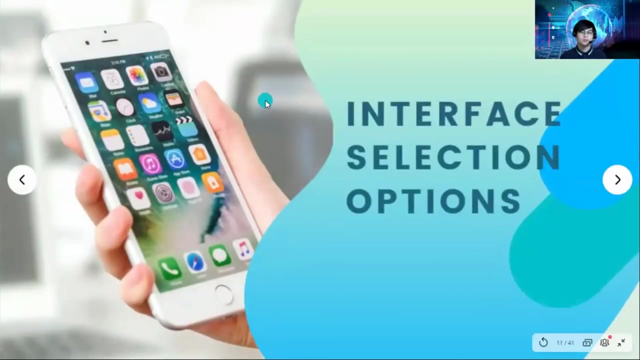 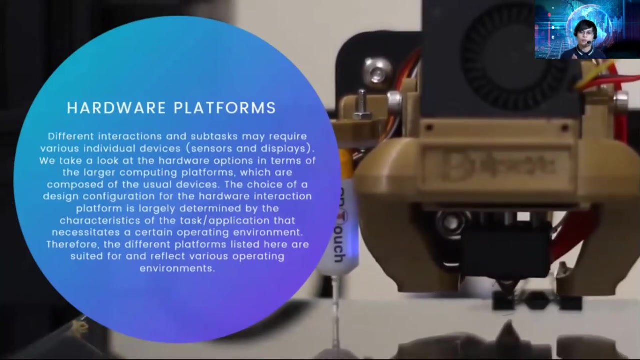 sensor and this application will be installed into a desktop or or in a mobile. no, so you must carefully think about the interface selection and consolidation. you consolidate, so as simple as that, okay. next the interface selection options. so what are different options in interface election? first is the hardware platforms? okay, so for the hardware platforms, different. 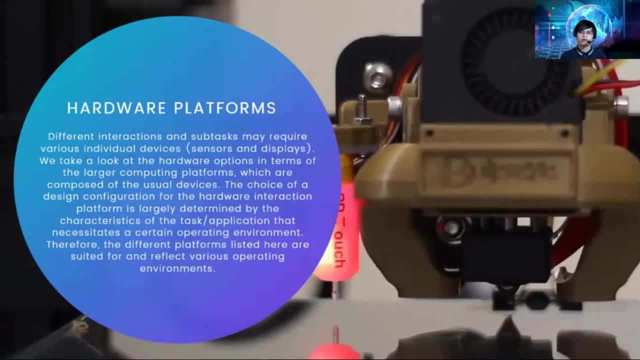 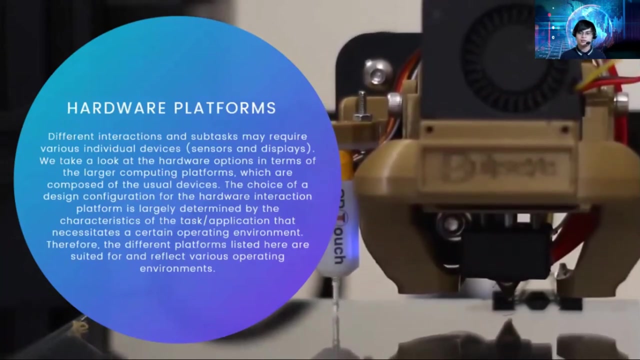 interactions and subtasks may require various individual devices, such as sample sensors and displays. we take a look at the hardware options in terms of the larger computing platform. the choice of a design configuration for the hardware interaction platform is largely determined by the characteristics of the task or 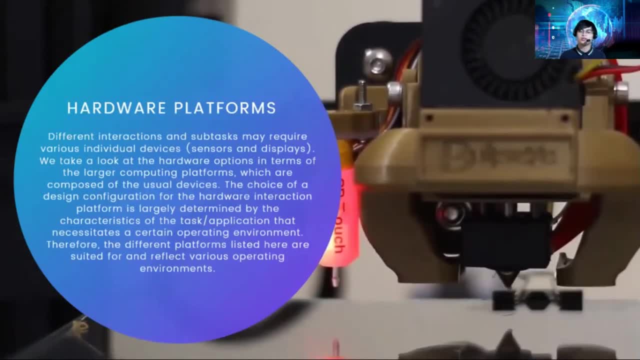 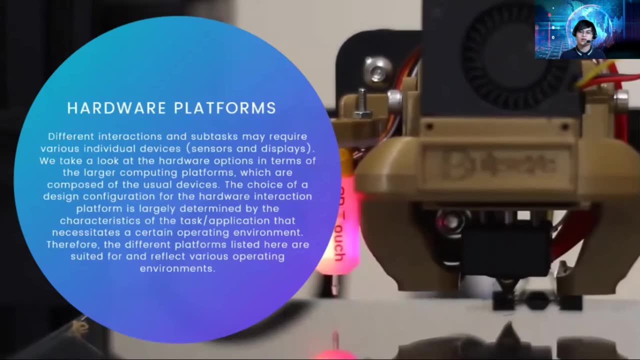 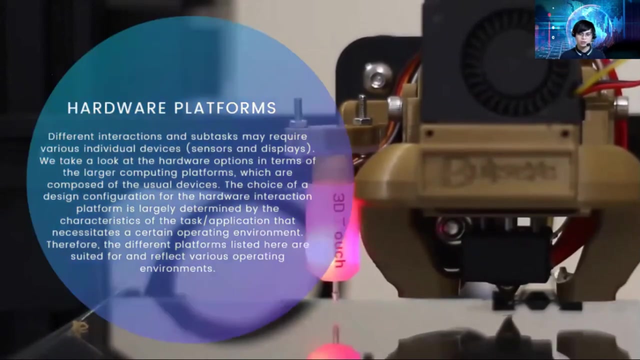 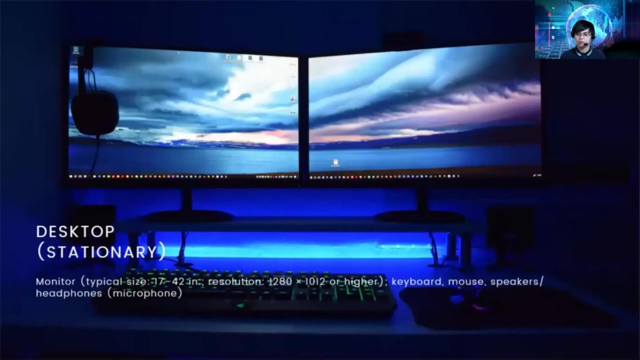 application that necessitates a certain operating environment. therefore, the different platforms listed here are suited for their reflect of various operating environments. so the hardware platforms includes different interface selection options and subtasks such as sample sensors and macro sensors and final estimator full ti set sampling and ensure while the interface is as easy to be integrated as possible. 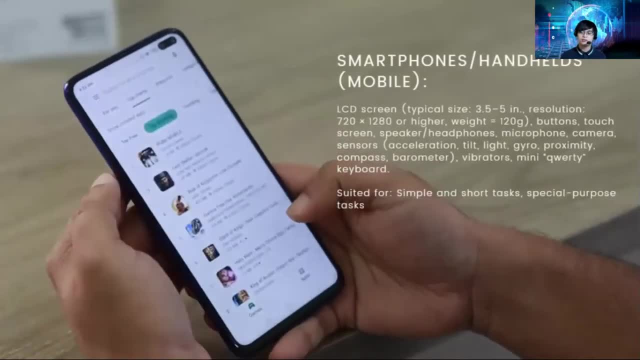 these are the key componentsные tools for understands those following: add 누구 of these elements icon. so enough volume, Iowa's. we need to add some supporting structures for a've highlighted using virtual characters and spoonfuls at the front of the desktop, as well as forming some common frames. thanks, 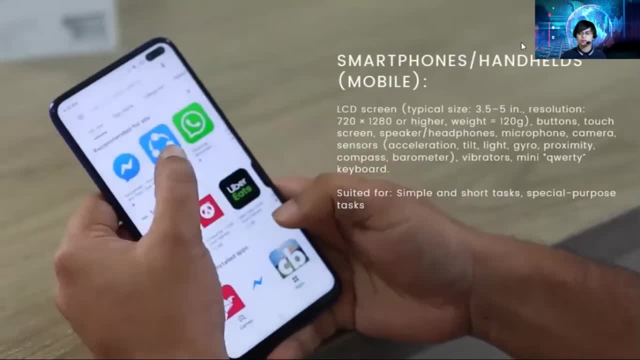 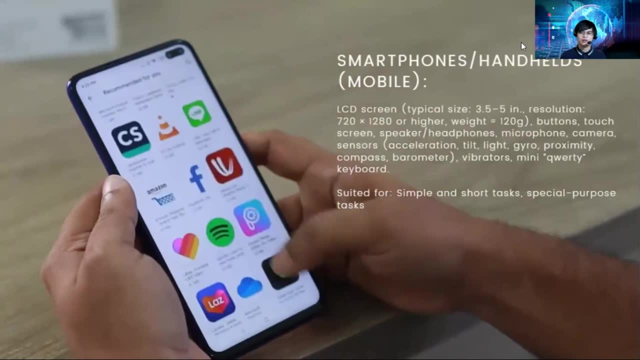 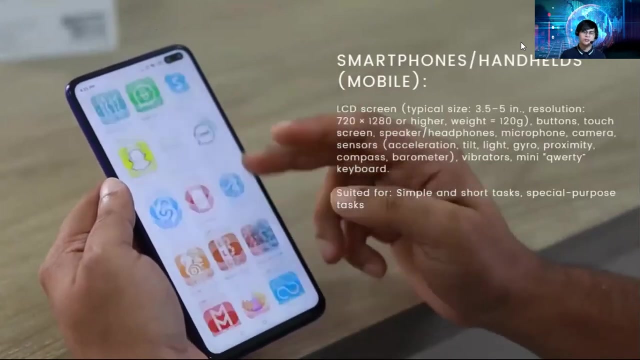 and there are three main components of Adapti, which are external softwares, and So it's a typical size of 3 to 5 inches, resolution of 722, by 1 to 80 or higher, Okay, And of course it has buttons, touch screens, speakers or headphones, microphone, camera, sensor, etc. 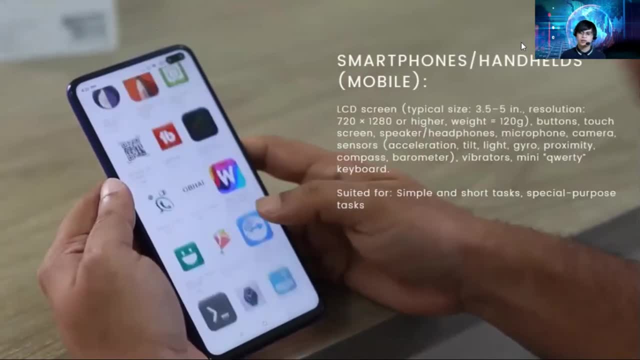 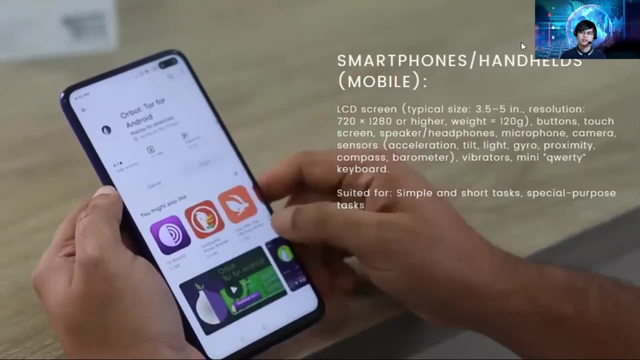 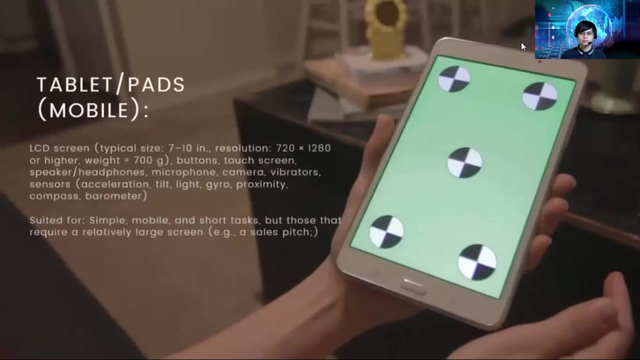 Okay, So smartphones are suited for the simple task. simple and short task, So special purpose task. So it's done And no need to further discuss. because smartphones no Kabalong nagin mo ana Tablets, Of course, nakakita na tag tablet no. 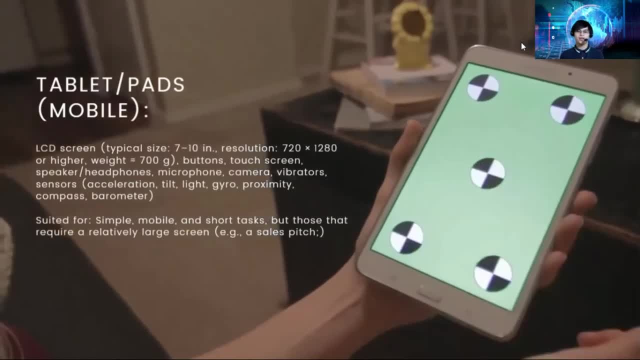 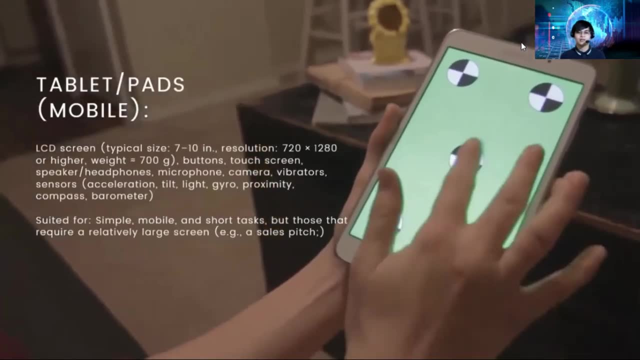 Kung wala tanaka unog tablet nakakita na tag tablet. Okay, So typical size is 7 to 10 inches, with a resolution of 720 by 1280 or higher. So again, mas dako siya sa tong smartphone. no. 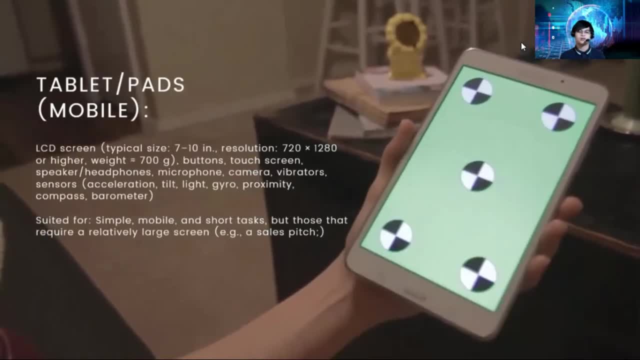 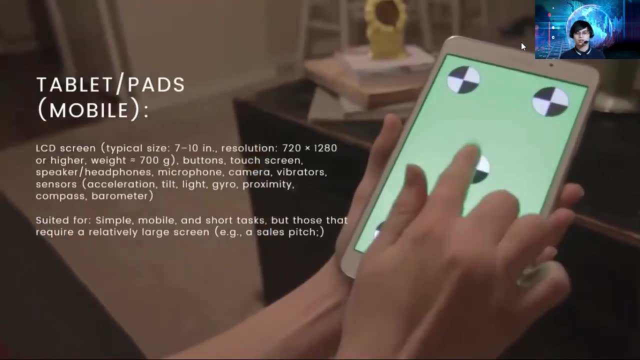 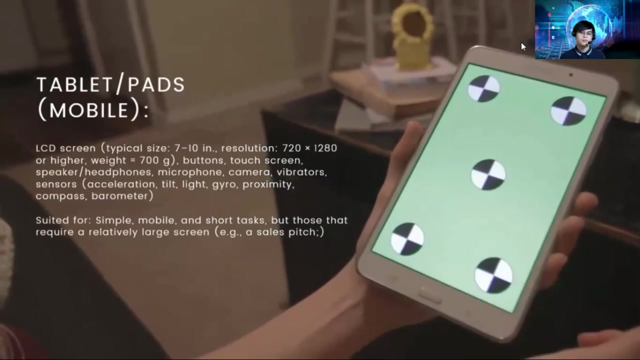 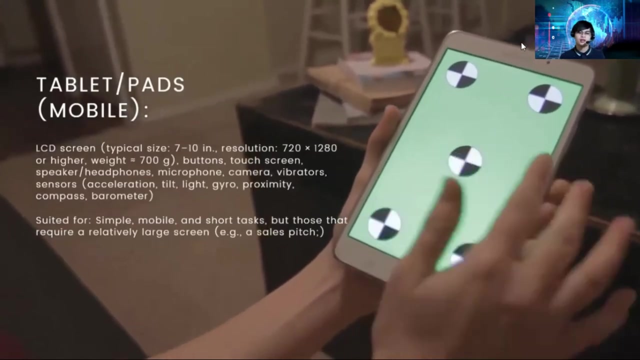 It also has spot-ons: Touch screens, speaker headphones, microphone camera, vibrators, sensors or acceleration, tilt, light, gyro, etc. Okay So, tablet is suited for simple, mobile and short tasks, But those that require a relatively large screen. 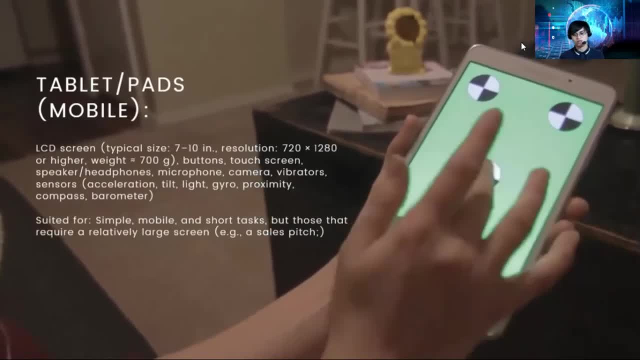 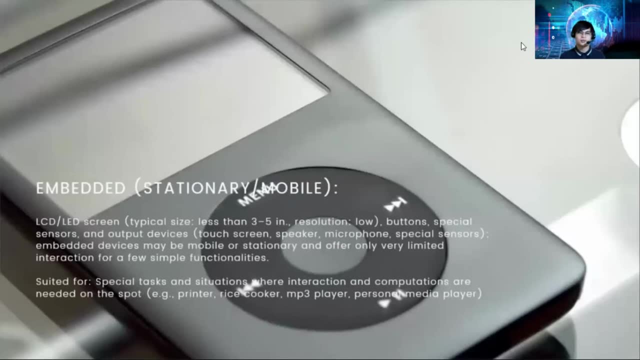 Okay, So example would be a sales speech. Next, We also have embedded, or stationary, or mobile, If you are familiar with- I don't know if naa pa ba ni karoon, no Yung mga MP3s, yung mga LED screens. 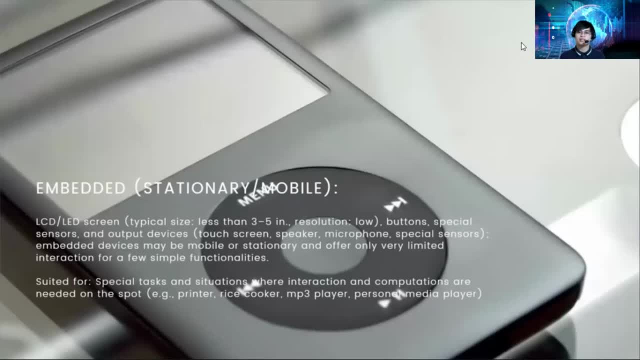 Okay, So typical size of less than 3 to 5 inches. Of course it also have spot-ons, special embedded devices or maybe mobile or stationary, And offer only a very limited interaction for a few simple functionalities. Okay. 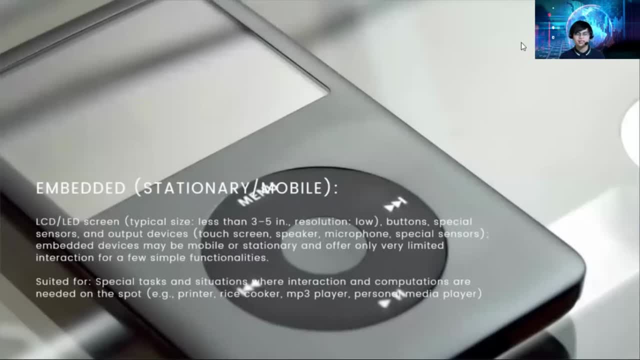 So it is suited for special tasks and situations where interaction and computations are needed on the spot. It should. example: we have printer, rice cooker, MP3 player, ya, the personal media player, Okay, Something like that. Next is the TV consoles. 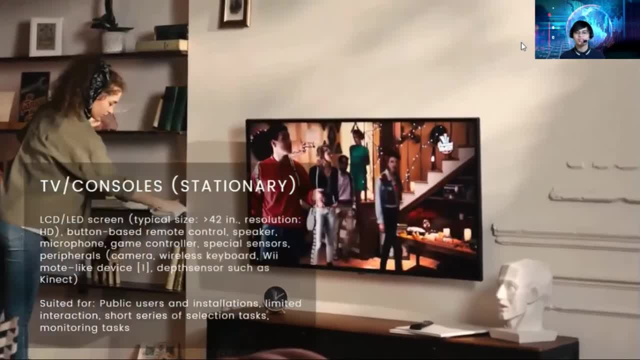 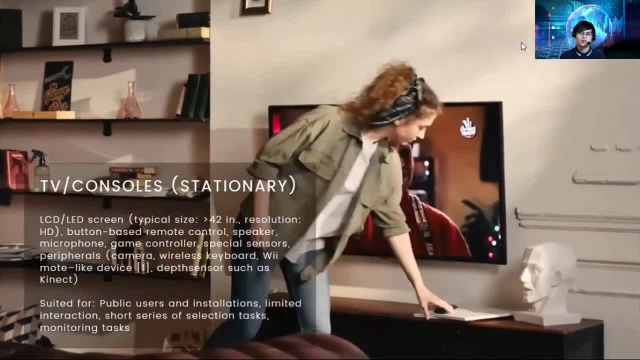 So it has a larger size of around 42 inches or less than So. it has a larger size of around 42 inches or less than It also. ah, it also has a remote, a button based, remote-controlled speaker, a microphone. 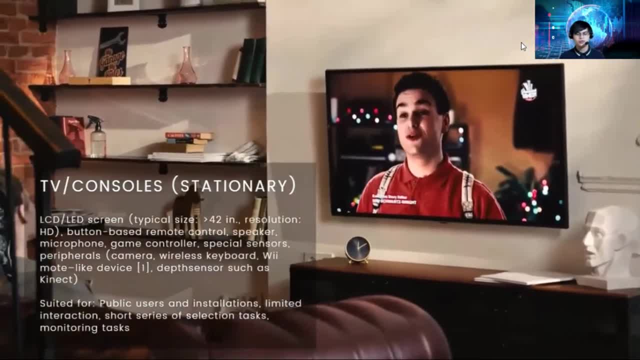 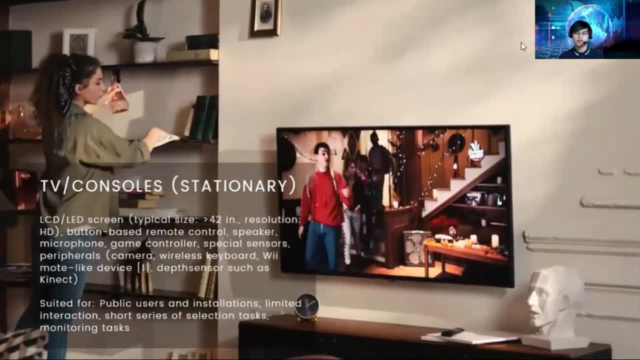 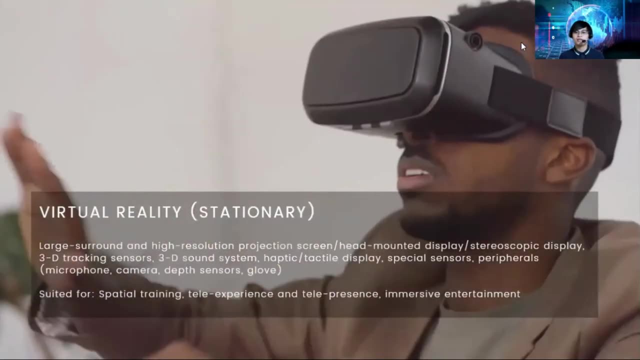 a game controller, et cetera. So TV consoles is suited for public users and installations limited interaction. So TV consoles is suited for public users and installations. limited interaction. short series of selection tasks and monitoring task. Okay, Next is the virtual reality. 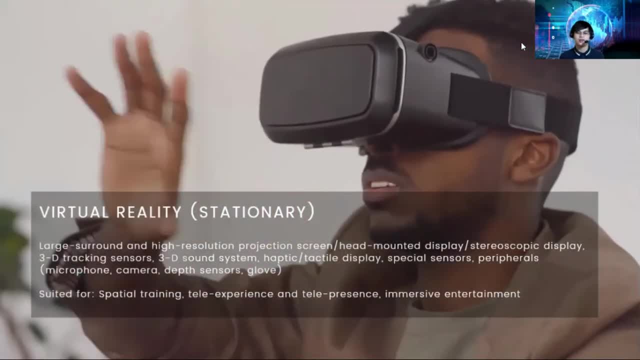 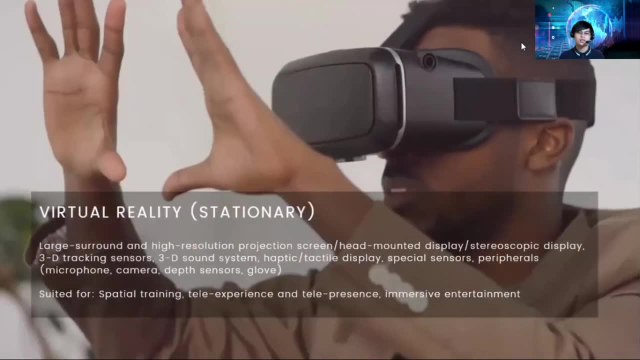 Okay, Okay, Okay, So it is a large surrounding. So it is a large surrounding round and high resolution projection screen, head mounted display, stereoscopic display, 3D tracking sensors, 3D sound systems, haptic or tactile display. 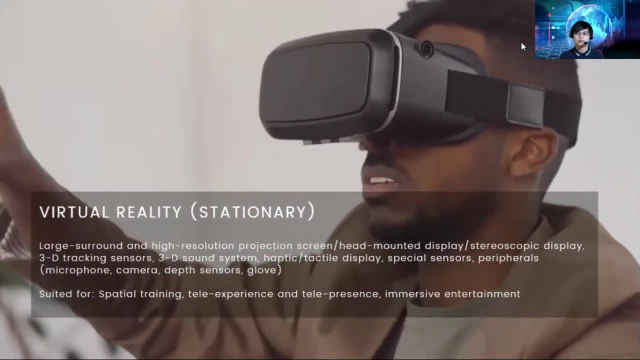 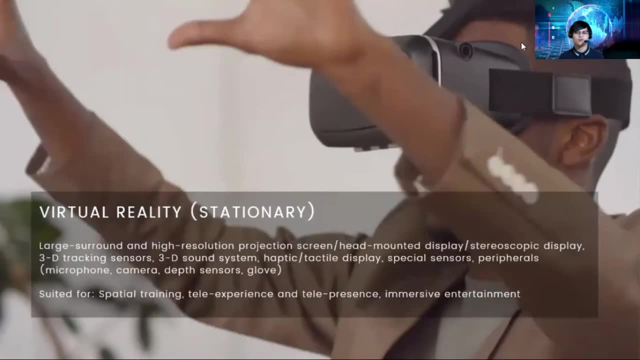 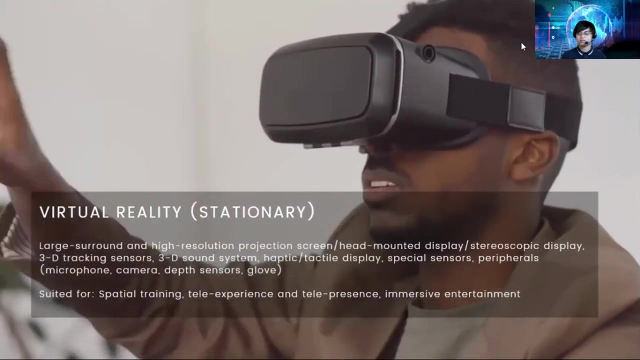 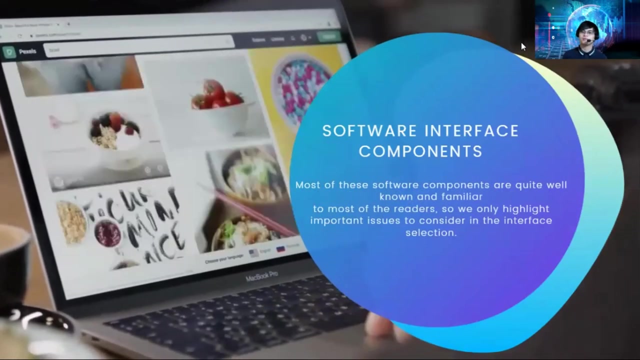 special sensors, peripherals: we have microphone camera, the depth sensors and glove. So virtual reality is suited for special training, daily experience and daily presence and an immersive environment. Okay, so those are the different hardware platforms. Now we're gonna move forward with the 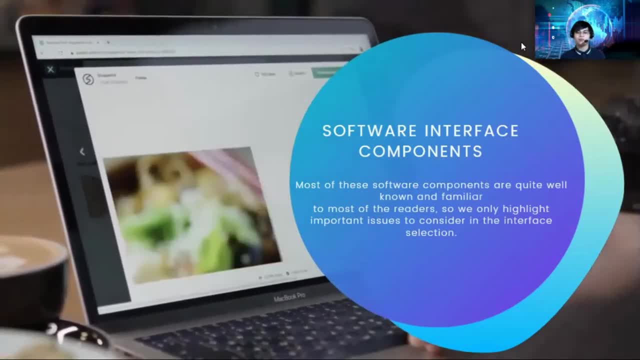 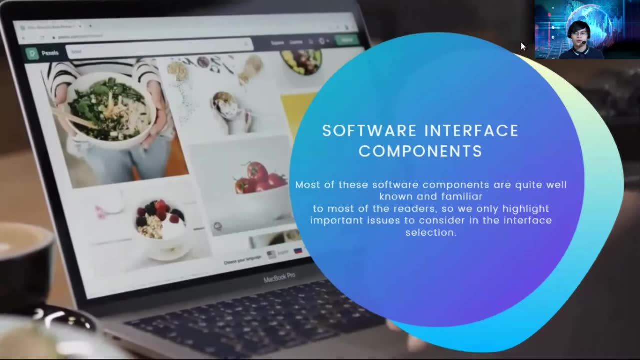 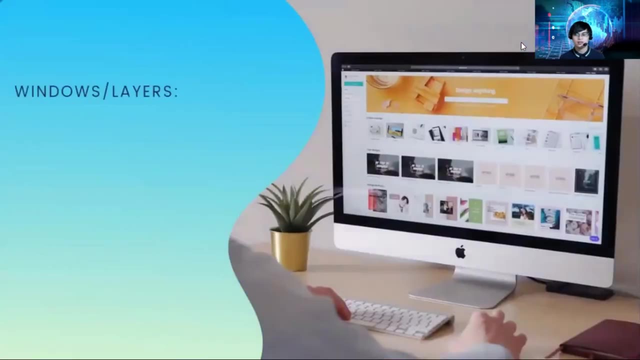 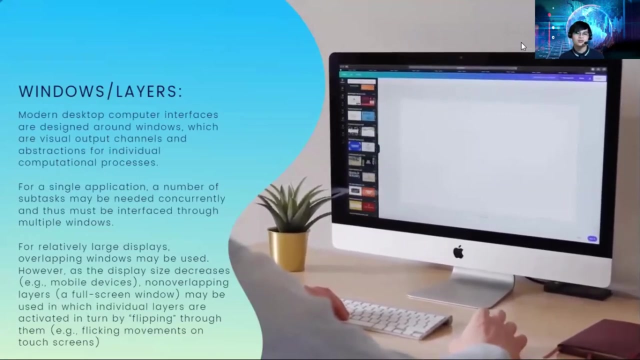 software interface component. Most of the software components are quite well known and familiar to most of the readers, so we only highlight important issues to consider in the interface selection. So what are the? this number one, windows or layers? modern desktop computer interfaces are designed around windows. 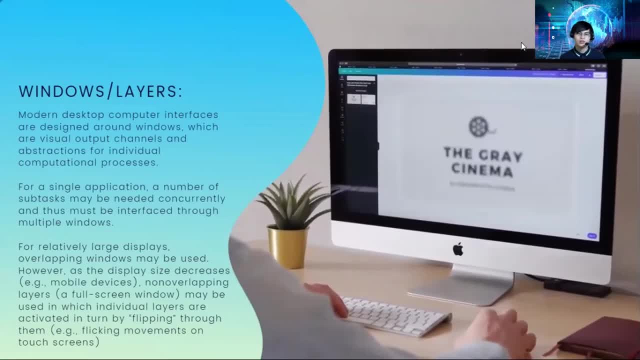 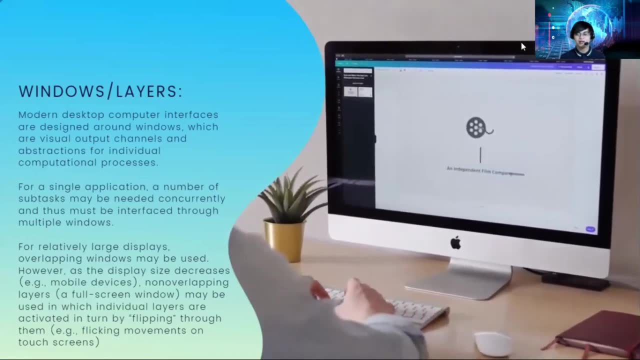 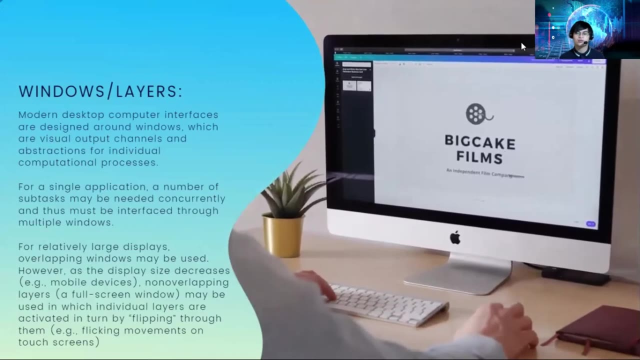 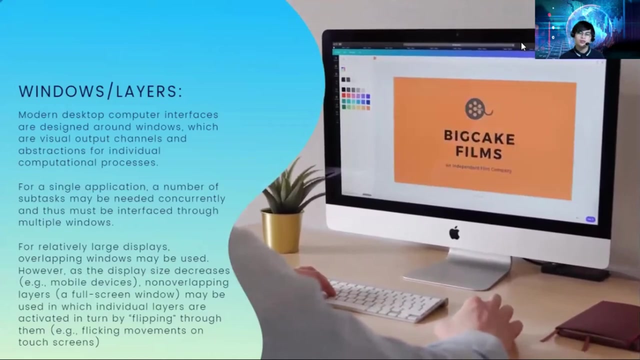 which are visual output, visual output channels and abstractions for individual computational processes. so for a single, single application, a number of subtasks may be needed concurrently and this must be interfaced through multiple windows. so for relatively large displays, overlapping windows may be used. however, as the display size decreases in the mobile devices, 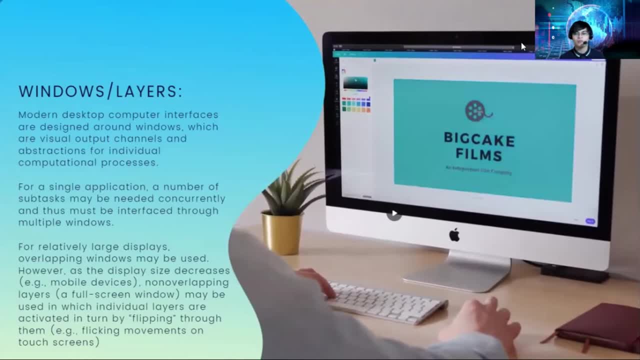 non-overlapping layers. a full screen window may be used in which individual layers are activated in turn by flipping through them, or example would be flicking movement on that screens. so, as you may have noticed, no, um, some of the conga brows brows mo, no, or this is a 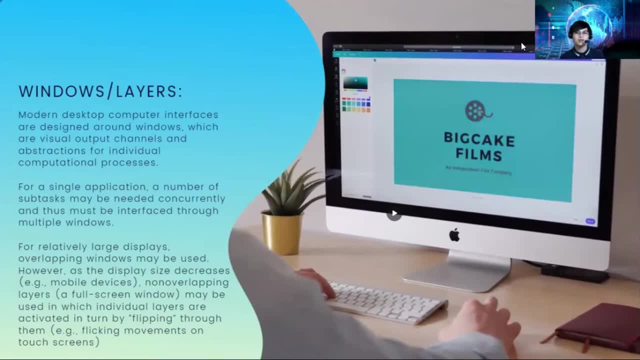 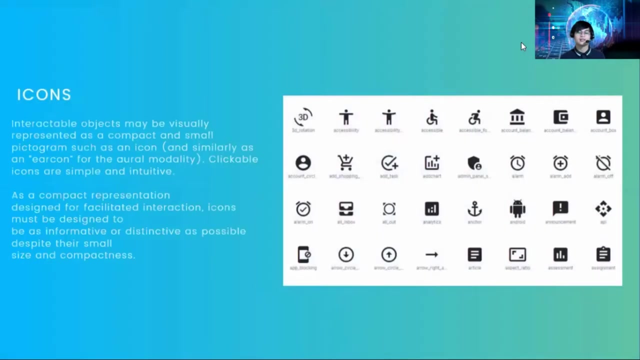 facebook. okay, there is a different ui design in in the desktop and then in the mobile. okay, so that is our. so we have the first component, windows or layers. next is the icons. okay, so icons or interactable objects may not may be visually represented as a compact and small pictogram, such as an icon. 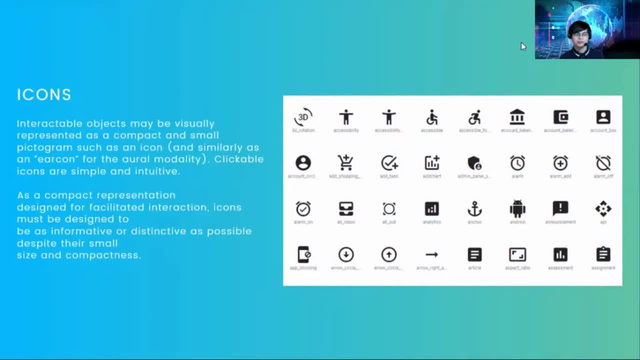 and similarly as an aircon for the oral modality. clickable icons are simple and intuitive, so, as a compact representation, they are designed for facilitated interaction. icons must be designed to be as informative, as distinctive as possible, despite their small size and compactness. okay, so we have these examples in 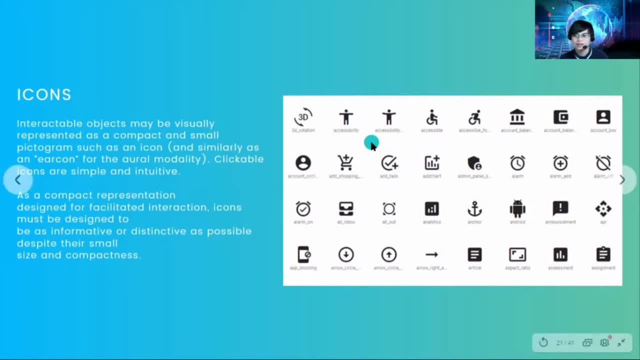 here, of course, if you've seen this sign um, i'll just give you an example. can you turn no, so it tells you that this, this is an alarm. okay, alarm on. or or an icon which is like this: so this is a shipping card, or this is a card, this is. 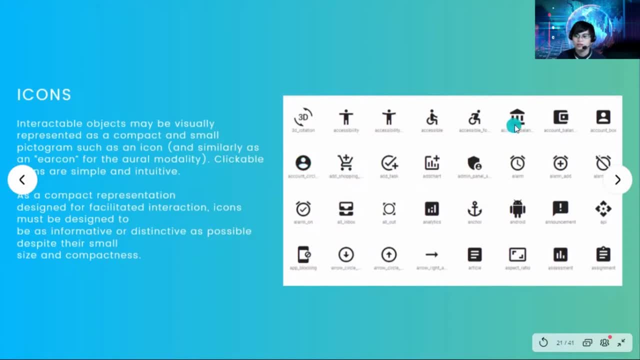 an account, no a profile, or this is a bank. okay, so those were some of of the icons that you can use when you develop a system or software, so you may use again an icons. if you have noticed, it's a facebook. they've got some mobile near. 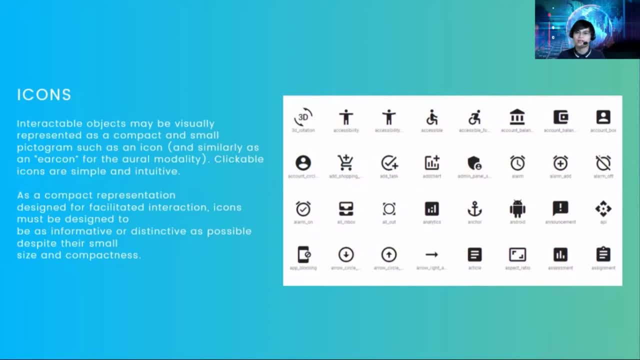 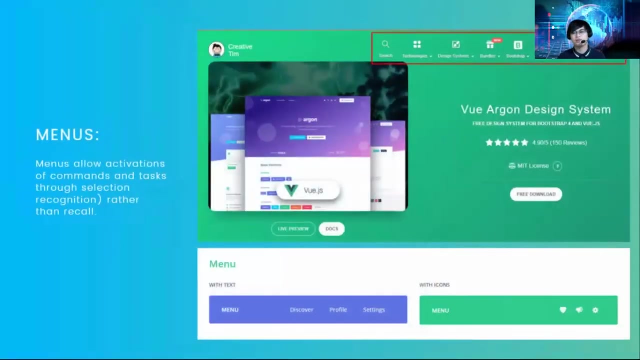 delete word on your home profile, not just your profile, but icons. icons in your newsfeed. icons are different videos on your new posts. okay, so, and next is very important, of course, all applications has menus. this is very useful for the user to, of course, navigate your system. 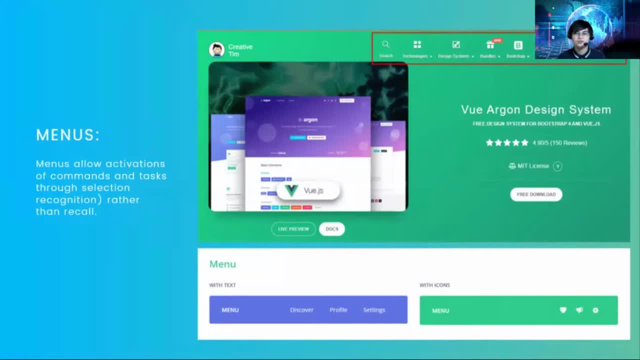 So these are allow activations of comments and tasks through selection, recognition rather than recall. So menu, menu bars, menu navigation, Let's say it's that So. example: if I want to navigate to the technologist's page, the search page, the bundles, etc. 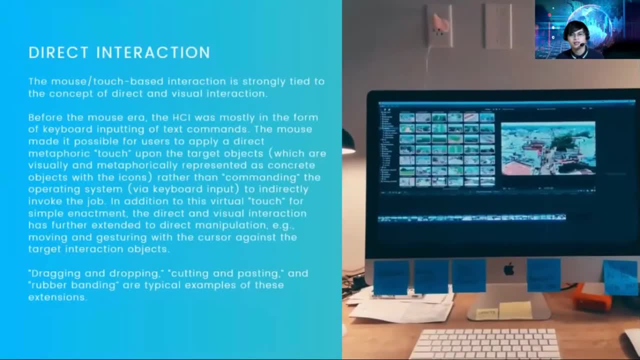 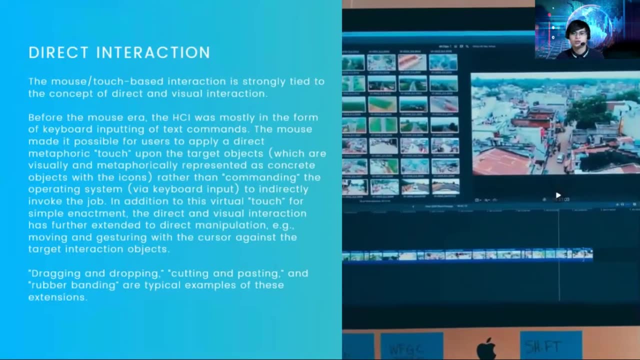 Okay, the menus or the navigations. Next is the direct interaction. So what is this direct interaction? The mouse or touch-based interaction is strongly tied to the concept of direct and visual interaction. So before the mouse era, the HCI was mostly in the form of keyboard inputting of text commands. 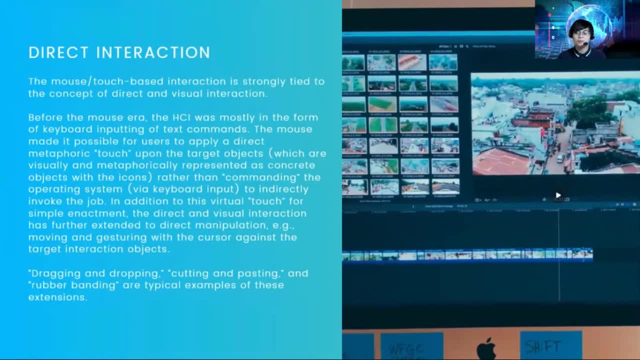 The mouse made it possible for users to apply a direct metaphoric touch upon the direct objects, which are visual interactions and visual interactions represented as concrete objects without the icons, rather than commanding the operating system via keyboard input to directly invoke the job. In addition to virtual touch for simple enactment. 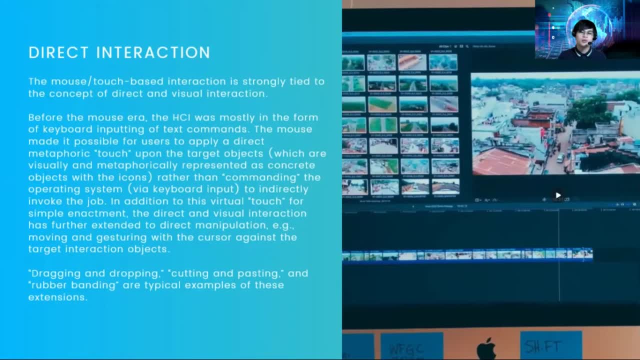 the direct and visual interaction has been further extended to direct manipulation: Up to 10 minutes' gesturing with the cursor against the target interaction object. So, for example, the dragging and dropping- okay, cutting and pasting and rubber banding are typical examples of these extensions. So, yeah, there is a direct interaction, Okay. 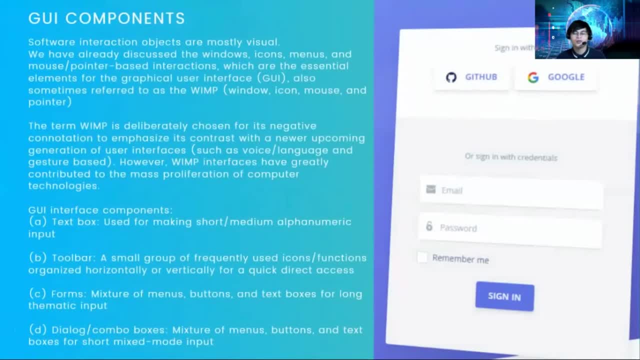 Next, the GUI components. Okay, of course we are very familiar with graphical user interface. You can see the icons, windows menus, etc. Okay, so software interaction objects are mostly visual. We have already discussed the windows icons, menus and mouse or pointer-based interactions, which are the essential elements for the graphical user interface. 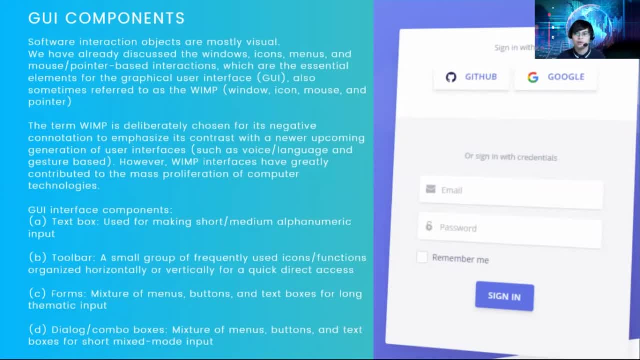 So also sometimes referred to as the WIMP or the window icon, mouse and pointer. So the term WIMP guys is deliberately choosing for its negative connotation to emphasize its contrast. So the WIMP is a way of using the digital interface to create a visual experience with a newer upcoming generation of user interfaces such as voice or language and gesture-based. 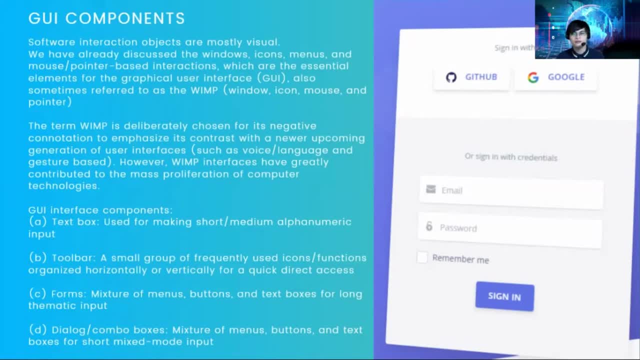 However, WIMP interfaces have greatly contributed to the mass proliferation of computer technologies. okay, So the different components of GUI is of course. we are very familiar with text box. It's like you can register and log in with a different text box. 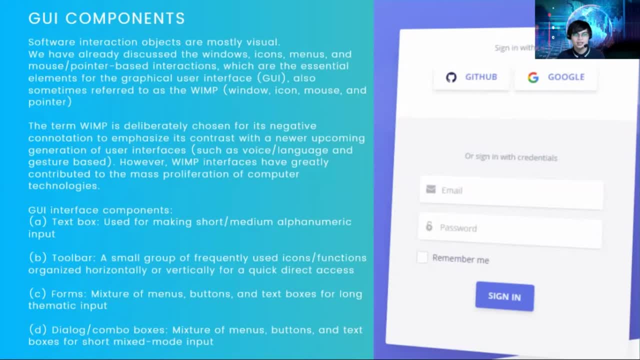 applications ago row. so not my login car, no, my type in casa among name, email and password. so I text back text box. sorry, tall bars. okay, the gamitans go to the moon. if you know how to make a Photoshop, Google Docs or Microsoft Word, Microsoft sheets, presentations, name, a total bars at us. 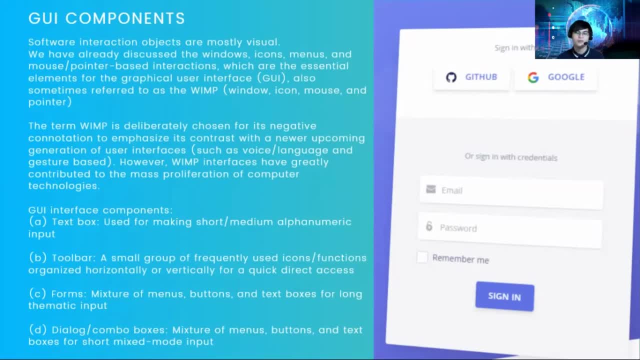 okay, so that's one of the GUI components. also forms: okay, very familiar. the mixtures of menus, portals and text boxes for long thematic input, and also dialog or combo boxes, normal models, a pillage data. this is a mixture of menus, buttons and text boxes for a short mixed mode input. okay, so let me give you an. 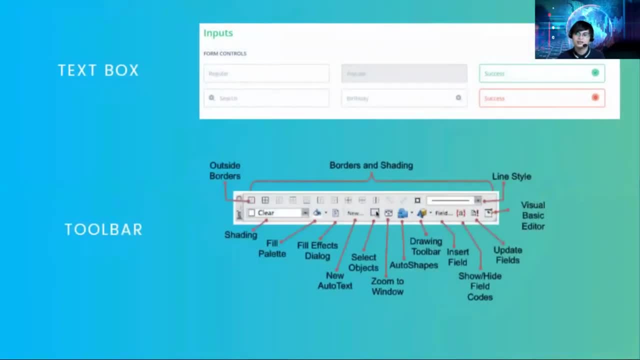 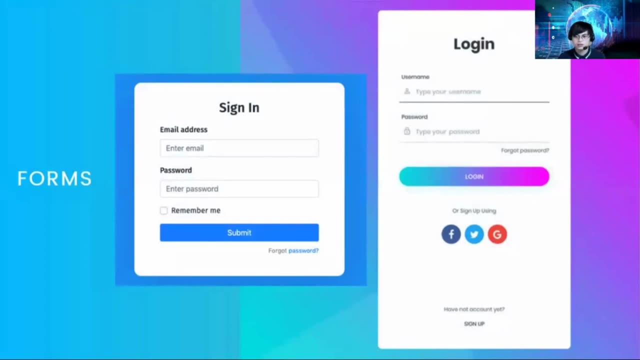 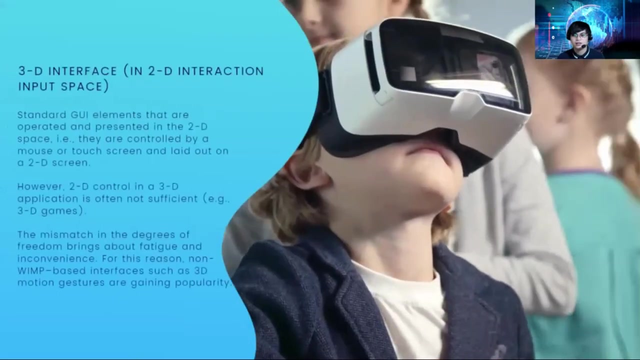 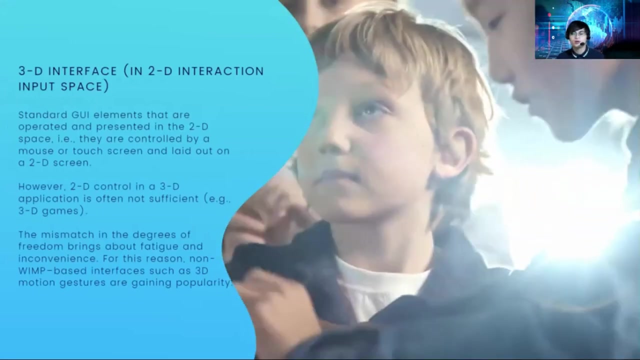 example. so text boxes for long thematic input. okay, so let me give you an example. so text box connection data toolbar and in then course, forms, and then we also have models. next is okay, the 3d interface into the interaction input space, so standard GUI elements that are operated and presented in the 2d space, or they are: 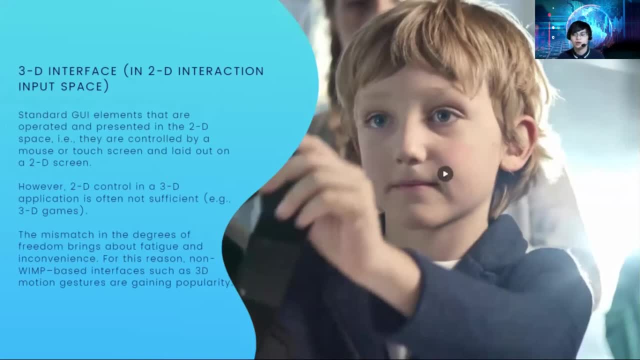 controlled by a mouse or touch screen and laid out on a 2d screen- okay. however, 2d control in a 3d applications is often not sufficient. there's great example: 3d games- okay. so the mismatch in the degree of freedom becomes brings about fatigue and 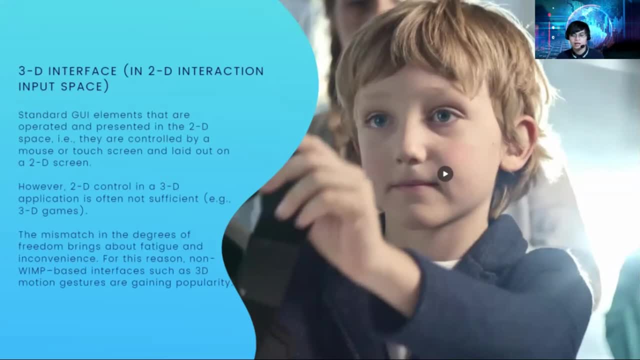 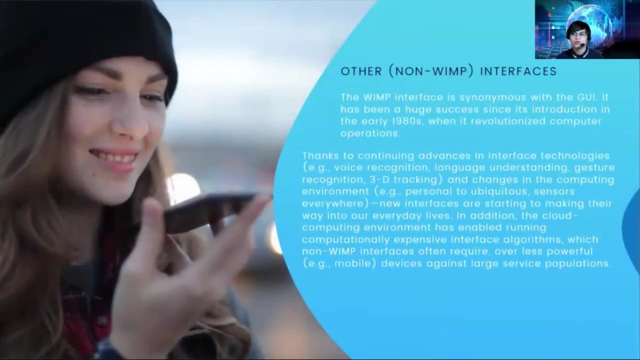 inconvenience. so for this reason, non-wimped based interfaces are such as 3d motion gestures are gaining popularity. okay, okay, the other non-wimp interface. so the wimp interface is synonymous with the GUI. so it has been a huge success since its introduction in the early 1980s. 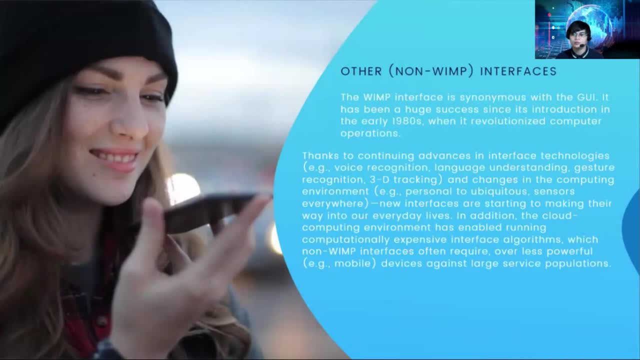 when it is revolutionized computer operations. so, thanks to the continuing advances in interface technologies- examples the voice recognition, language understanding, gesture recognition or 3d tracking, and changes in the computing environment, samples, the personal to of you, shoes, sensors are everywhere- new interfaces are starting to making their way into our everyday lives. so in 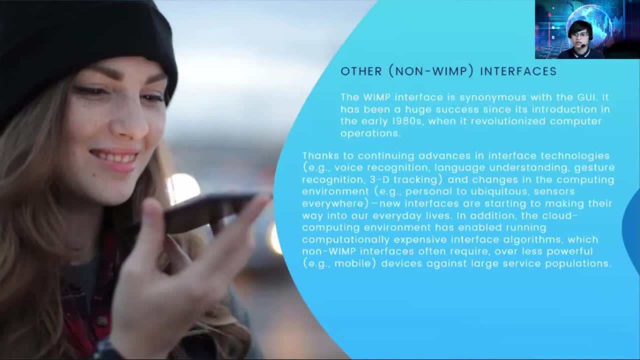 addition, the cloud computing environment has enabled running computationally expensive interface algorithms, which non-wimp interface often require, over less powerful in the mobile devices against large service populations. okay, so that is the non-wimp interfaces. okay, so again examples, be you know, the voice recognition on the language understanding, gesture recognition or 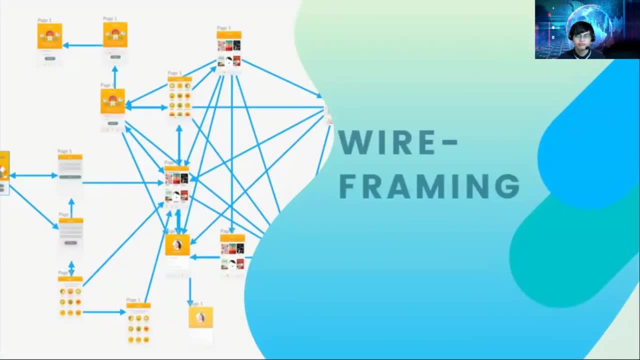 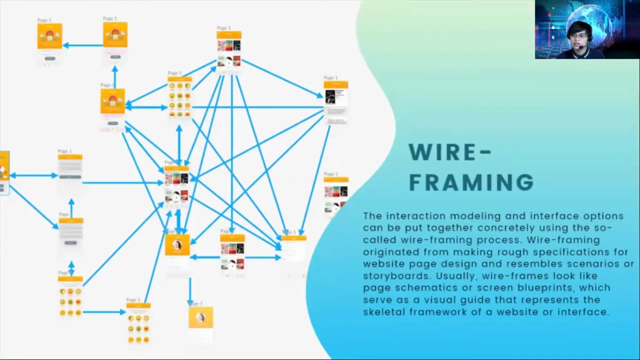 3d tracking, something like those things. O okay. next is when you design an application is: let's move with the wire framing. okay, in the wire framing. why is it important? the interaction, modeling and interface options can be put together concurrently using the so called wire framing process. so wire framing originated from making. 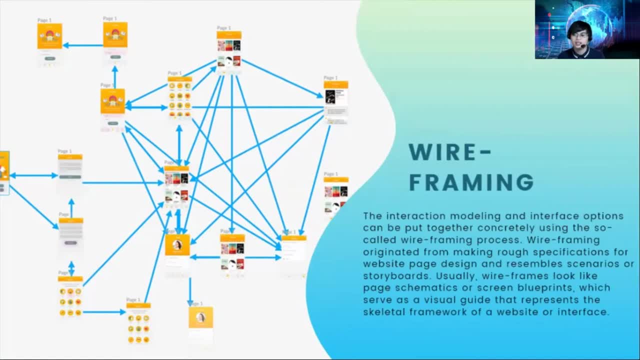 rough, so wire framing originated from making rough, so wire framing originated from making rough specifications for website page design and resembles a scenarios or storyboards, or wireframing, also called smack ups. no, so usually wireframes look like page semantics or screen blueprints, so which serve as a visual guide that represents 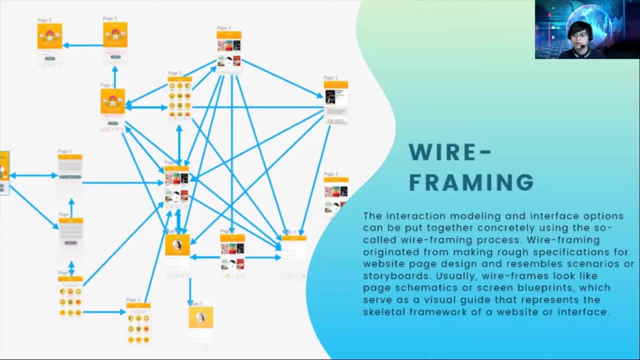 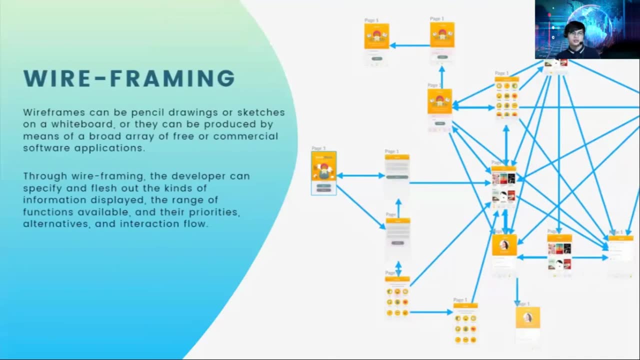 the skeletal framework of a website or interface. okay. so mag drawing, drawing, Connie, okay. wireframes can be pencil drawings or sketches on a whiteboard, okay. or they can be produced by means of broad array, array of free or commercial software applications. so there are, don't worry guys, cuz so wireframing the parts. 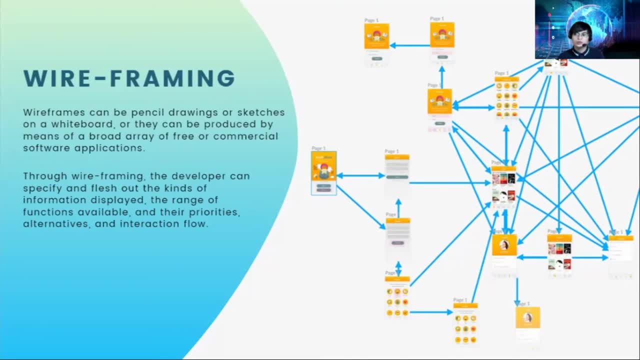 in your system. we'll be using a tool. no, but as of now, Kong Billy mama, access a ton of tools in your that I will be giving to you. you can feel free to just draw it in a, with you know, pencils or once a mongo. so the 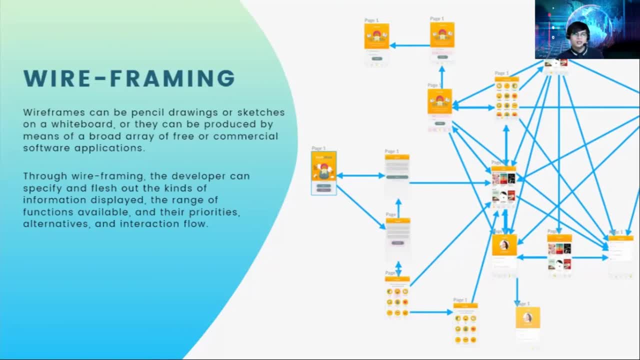 meter. okay, so again, the purpose of this? it is through wire framing, the developer can specify the flesh out of the kinds of information displayed, the range of the functions available and their priorities, alternatives and interaction flow. didn't do Makita Nia, the market as a developer? ah well they. 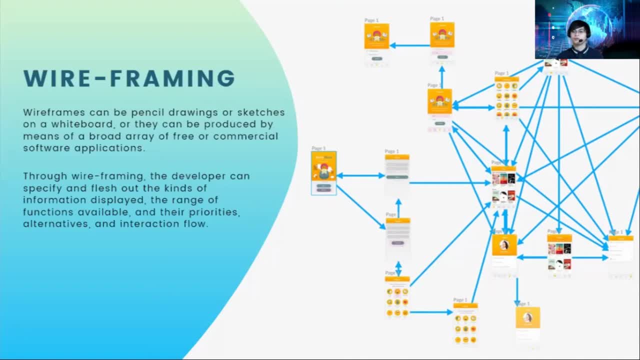 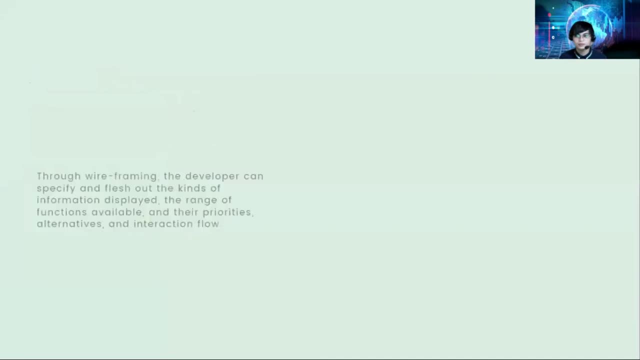 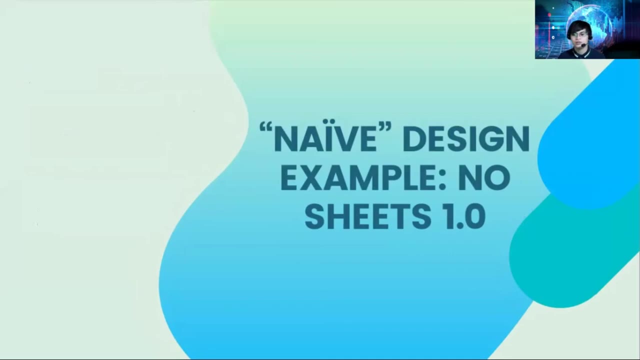 need a possible meta boss Ananga software. okay, so this is one of the most important also. okay, so now let's move on with the naive design examples. number no: sheets 1.0. actually. okay, so this is now the application of those design process. okay, let's take a look at this example. 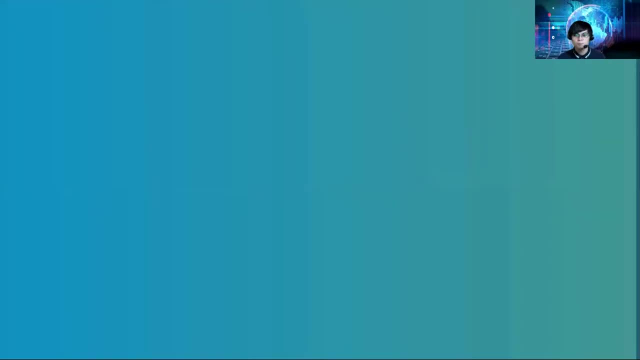 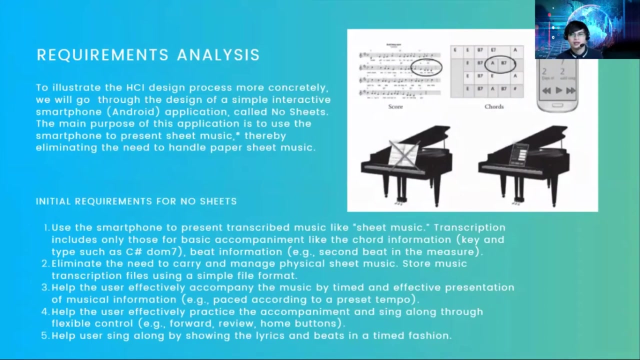 okay, so I'll like this first. okay, so, second image, so you can guess. okay, so, all right, let's take a quick look. okay, let's make a Turtle, and most now let's take this one. why am I still a quiteити okayamy out of the application? third zoot. 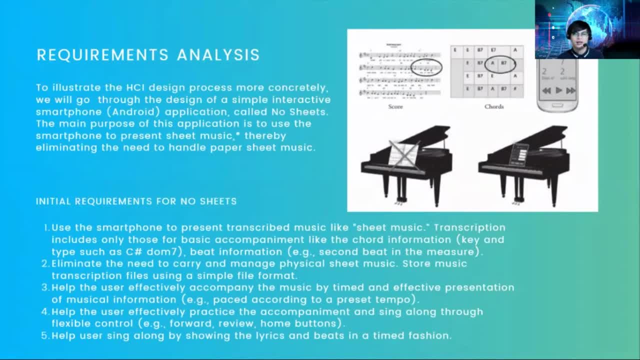 sheet music, Thereby eliminating the need to handle paper sheet music sheet. What I'm gonna take pronounce of shit. So initial requirements for no sheets, okay. So first, of course, use this smartphone to present transcribe music like sheet music. Transcription includes only those for basic accompaniment, like the chord information. 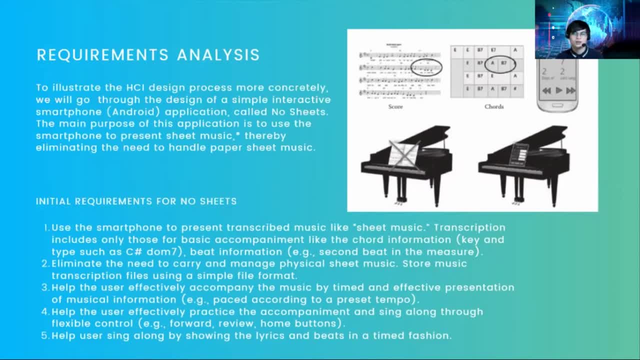 key in types such as C sharp dome, 7 bit information and Yeah example sound bit in the measures. and then also we eliminate the need to curry and manage physical sheet music. so store music transcription files using a simple file format and Other requirements should be help the user. 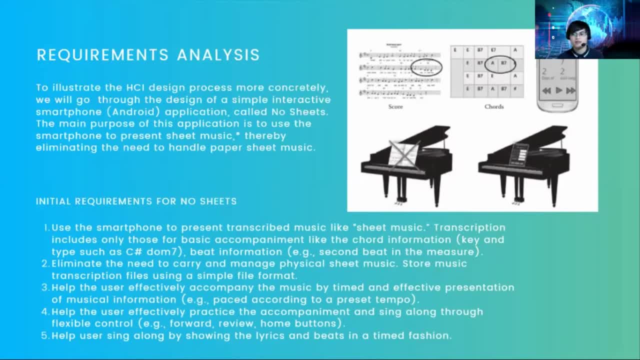 effectively accompany the music by time and effective presentation of musical information. and And help the user to effectively practice accompaniment and sing along through the flexible control. and Also will help the user to sing along by using the lyrics and beats in time fashion. So those were. 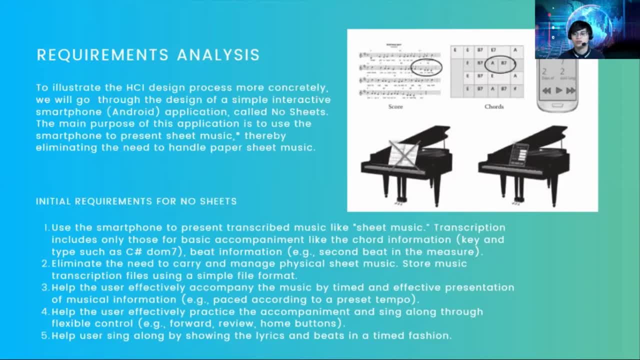 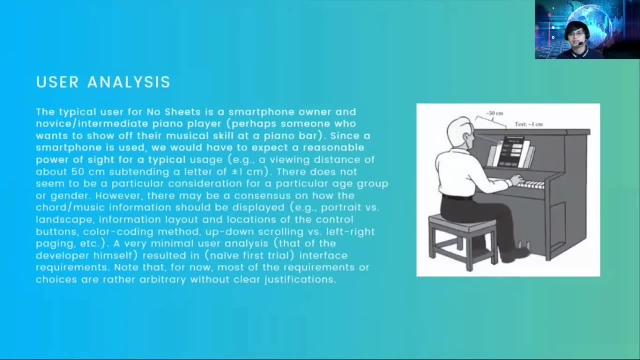 sample initial requirements for this application for the new search application. Next is the user analysis. okay so, So the typical user for no sheets is a smartphone owner and No voice or intermediate piano player: Okay so, perhaps someone who wants to show off their musical skill at the piano bar? 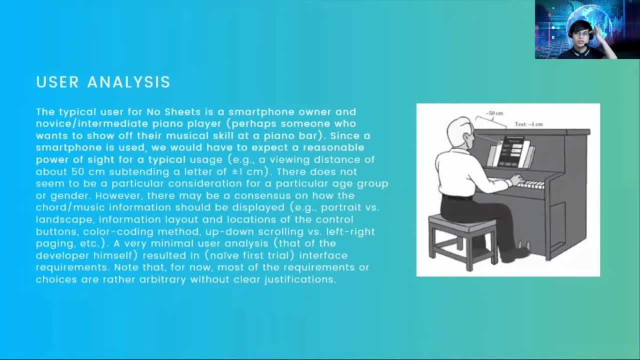 Since a smartphone is used, we would have to expect a reasonable power of sights for a typical usage. Okay, example: a viewing distance of about 50 centimeter subtending a letter of passage. Negative, negative one centimeter. Okay, so there does not seem to be a particular consideration for a particular age group or gender. 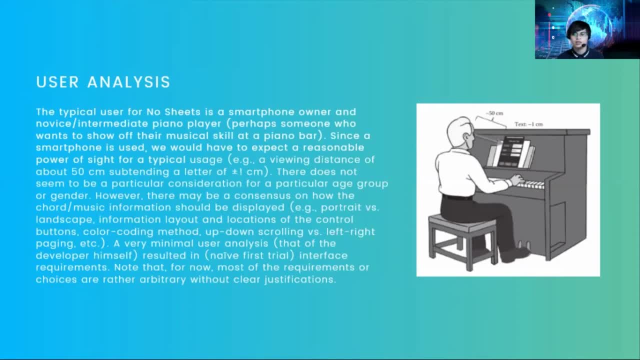 however, There may be a consistent consensus on how the chord or music information should be displayed, example, in portrait versus landscape information, layouts and locations of the control Paging, something like those things. the color coding method- Okay, the up-down Scrolling versus the left right paging- Yeah a. 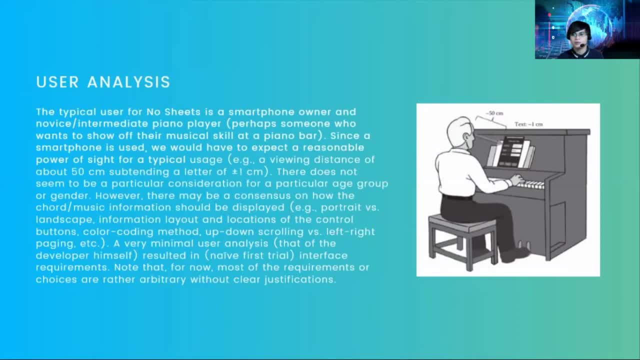 very minimal user analysis that of the developer himself resulted in, or a naive first trial interface requirements. So note that for now most of the requirements or choices are rather arbitrary, without clear justifications. So for the user analysis there is one chapter. for the- Yeah, this will be a. 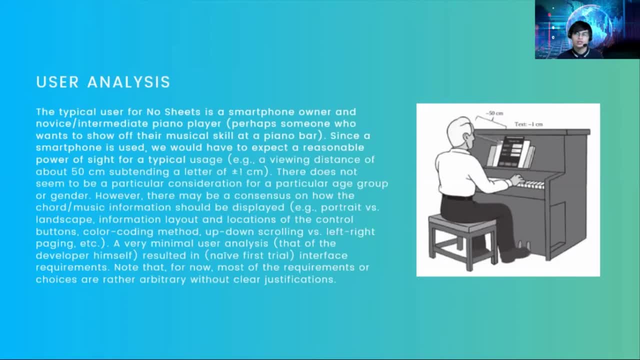 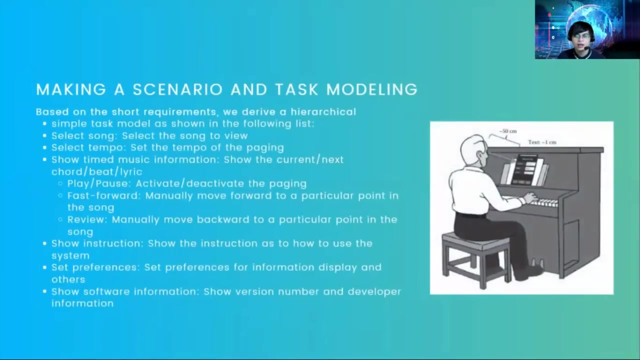 I Discuss further in the next chapter on how to really analyze- No So the users. a more application. That is one of our example. for now, Okay, and after that, okay. after not donation, analyze you, we will move to making a scenario and task modeling. so in here, based on this short requirements, we derive an a. 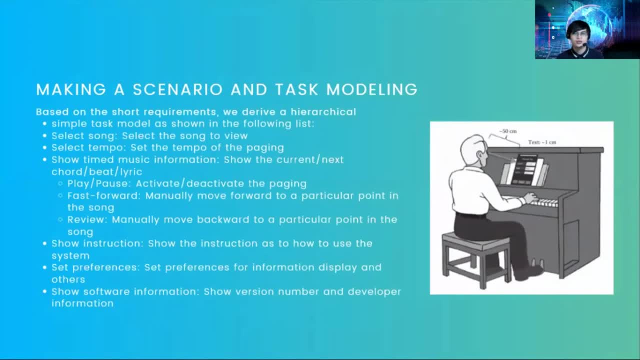 Error recall simple task model shown in the following list: Okay, first is select song. Okay, so the user were we're going to select a song, So there should be a select the song to view. Okay, Next is select tempo, So set the tempo of the paging. 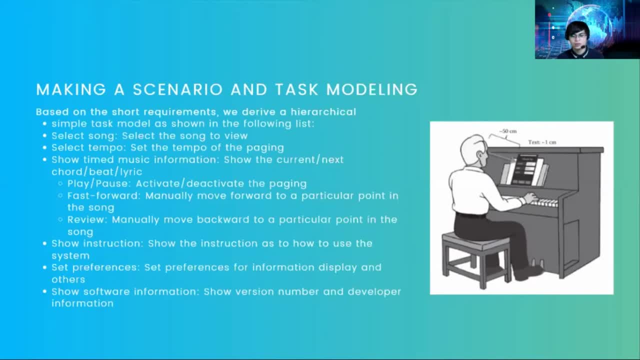 next next scenario or the task could be: Showtime, music information or show the current and next chord Or beat or lyric, Okay, and then we have the play and pause, the fast forward, the review and then the show instruction, or show the instruction as To how to use the system. 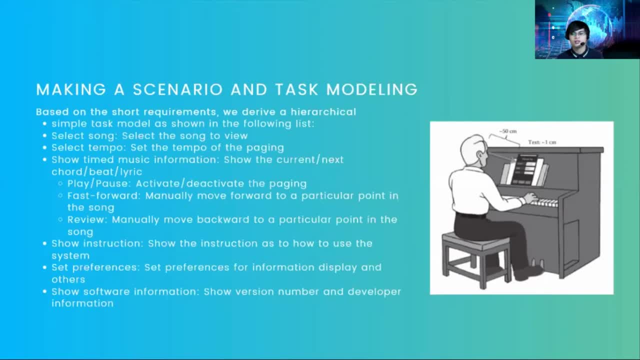 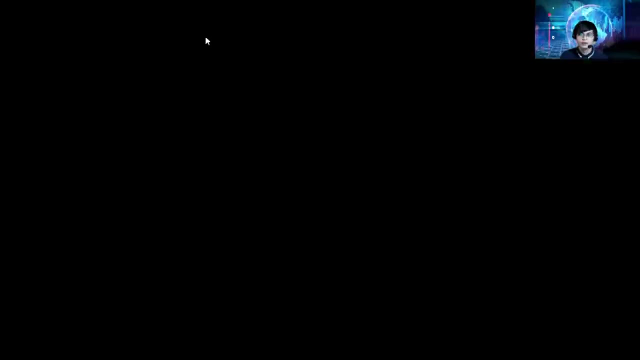 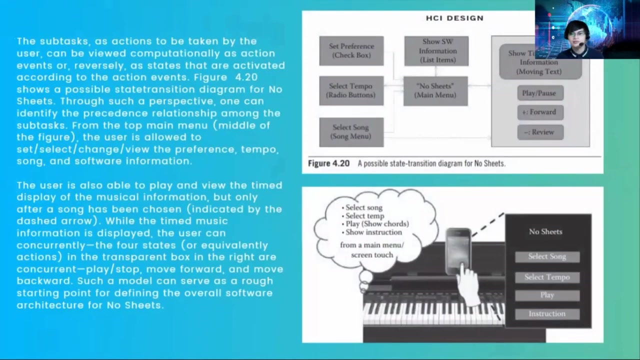 Okay, and set preferences. set preferences for information display and others and show information, software information, or show version number and developer information. So these were samples on the Notion's applications. okay, and then okay. okay, the subtasks, as actions to be taken by the user can be viewed computationally as action events or reversely states that are activated according to the action events. 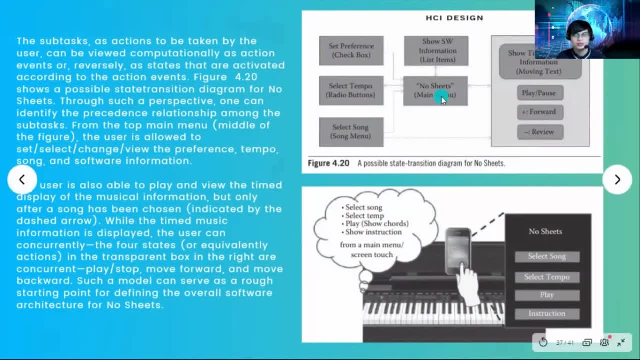 Okay. so as you can see here in our example, it shows a possible state transition diagram for Notion's. okay, so this one. Through such perspective one can identify the precedence relationship among the subtasks from the top main menu. 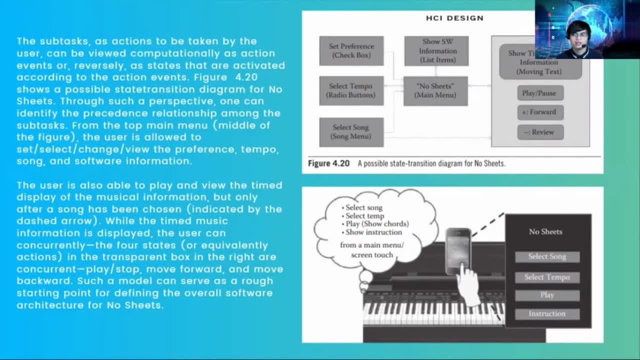 The user is allowed to. you know, set, select, Change, view the preference tempo, song software information. okay, so the user is also able to play and view the time displayed to the musical information, but only after a song has been chosen. you know or other could be. while the time music information is displayed, the user can concurrently the four states or equivalently actions in the transparent box in the Notion. 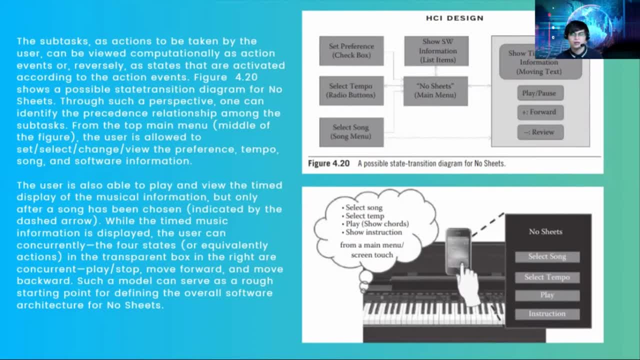 The right are concurrent. they can either play or stop, move forward and move backward, So such a model can serve as a rough starting point for defining the overall software architecture for Notion's. So take a look at this example. 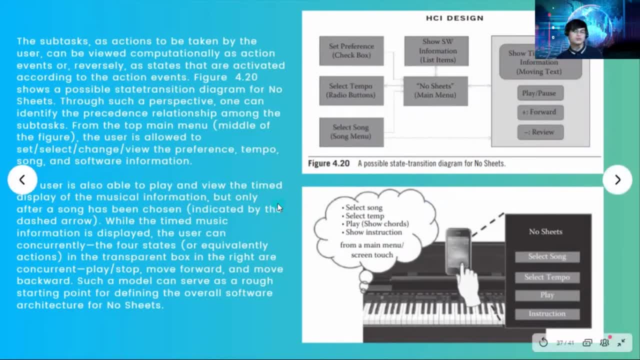 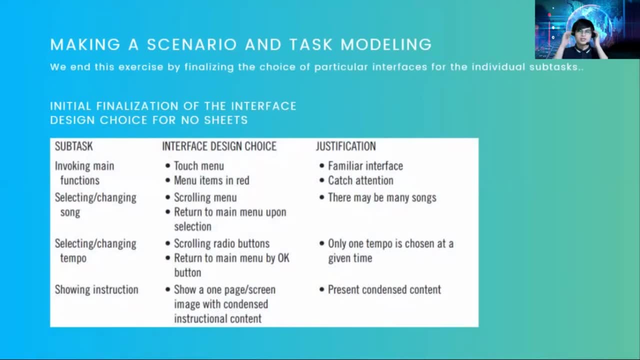 So here's this. one Number of you know models. yeah, Okay, so this is the initial. This is the initialization of the interface design choice for Notion's. So you define the subtask, the interface design choice and then the justification. 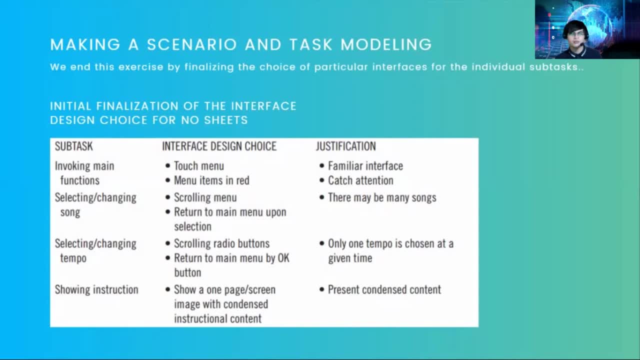 Okay. so let's say, for example, the subtask is invoking main functions. So in the interface design choice you have this touch menu, menu items and then in justification you know the familiar interface and then the catch tension. 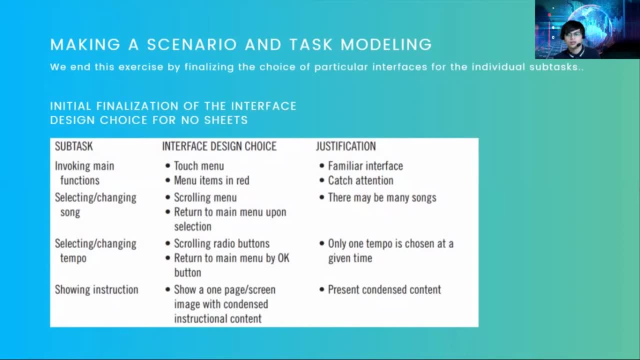 Okay. so in selecting or changing a song, Of course there is a scrolling menu. There's a return to main menu upon selection And then in selecting or changing tempo, there is a scrolling ready buttons. return to main menu by okay button. 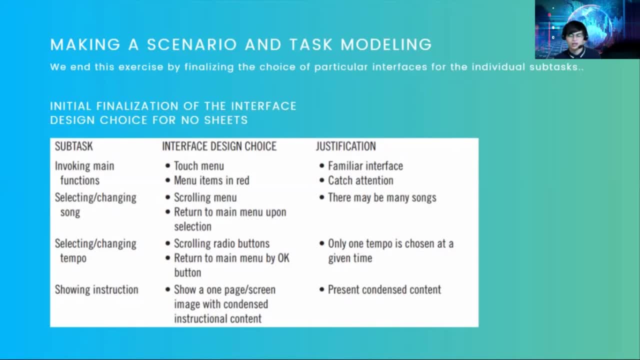 Only one tempo is chosen at a given time as the justification And also the task of showing the instruction. what will happen? it will just show a one-page screen or image with a condensed instruction. So that's the main screen that will be used for the instructional content. 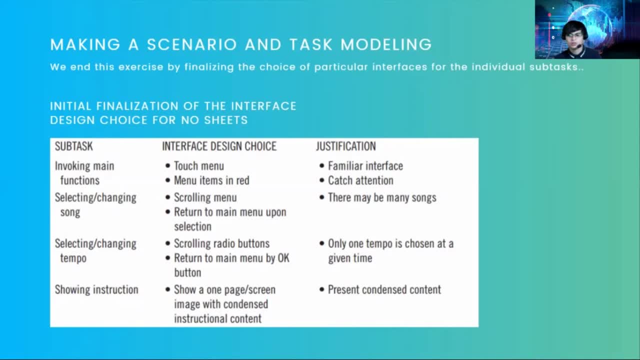 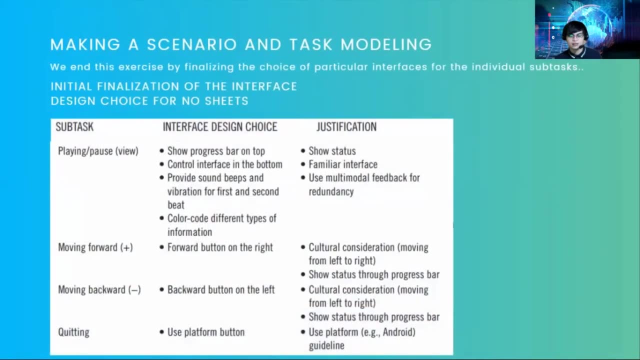 And as for the justification, it will present condensed content, So something like that. Okay, so in playing or pause, what we're going to happen will be: it will just show the progress bar on the top. control interface in the bottom provides sound beeps and vibration first and second. 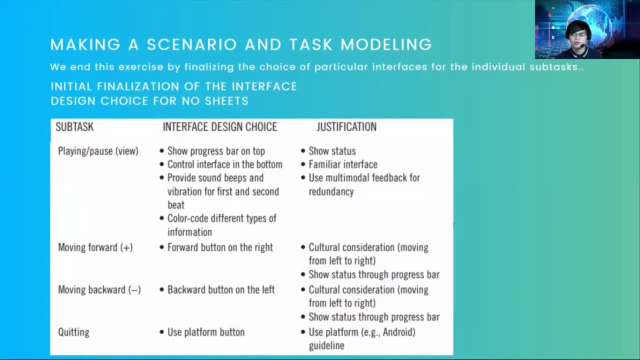 So guess this is just an example. Now you define what are the different tasks, task of, again, of your application. so with that task, once I am Akita didn't say user, no, okay, again you do the wireframing and then you do making. 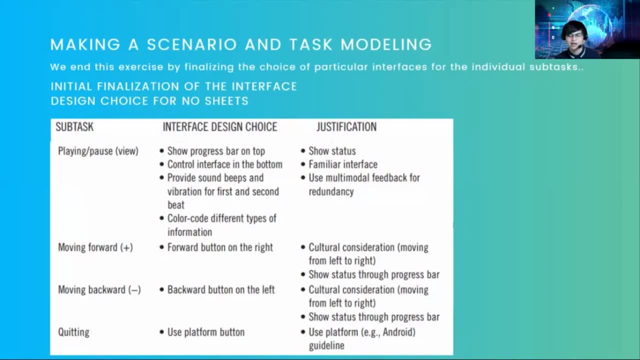 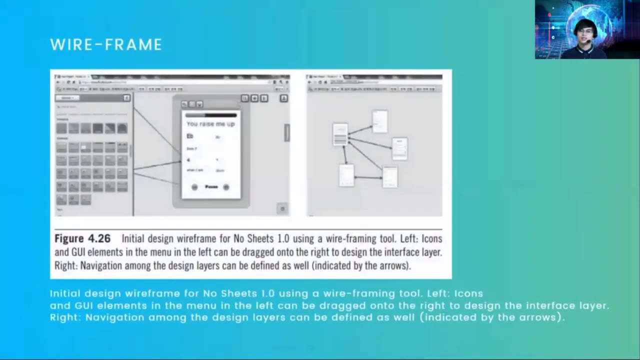 scenarios and task modeling. you stay down, you list down on. once I made a book. come on me, I mean I'm only on task as a design- the pot and Asha- okay. so next is the wireframing- okay. so this is one of the example. initial design wireframe for 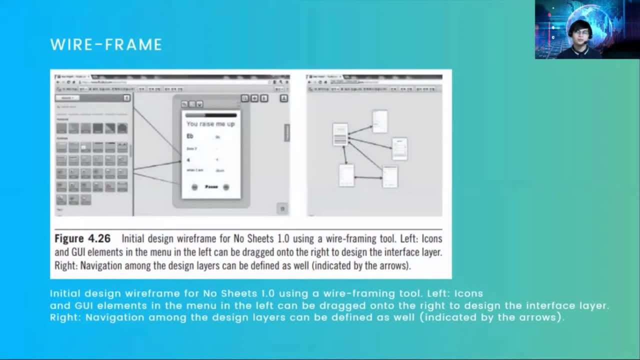 no sheets using a wireframing tool. okay, I will be giving you a wireframing tool. they don't want if you're not able to access, guy made you. is it bomb on a home? so don't worry, you can use pen and paper. so in the left icons and go away. 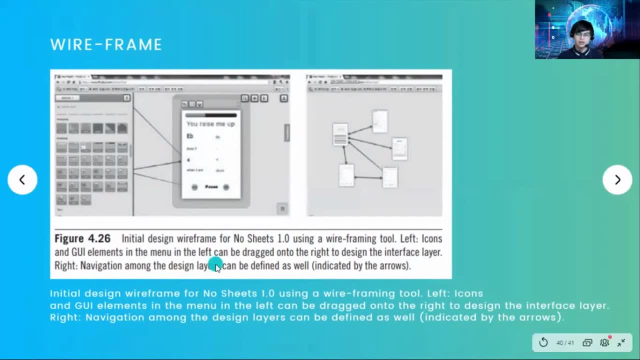 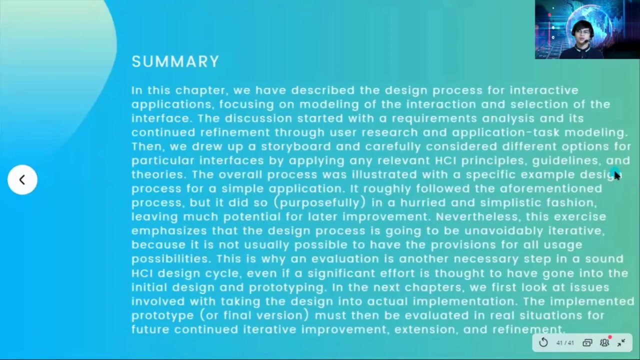 elements in the main menu that can be dragged, and to the right to design an interface layer: okay, and navigation among the design layers can be defined as well. so initial is an wireframe for no sheets using a wireframing tool. this one, okay. next, ok, no. 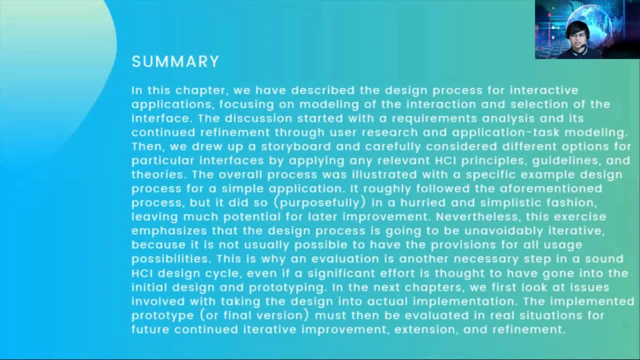 � no no everyday no no task modeling and then we drew up a storyboard and carefully considered different options for wait for particular interfaces by applying any relevant HCI principles guidelines and theories so the overall process was illustrated with the specific example design for a design process wait for a 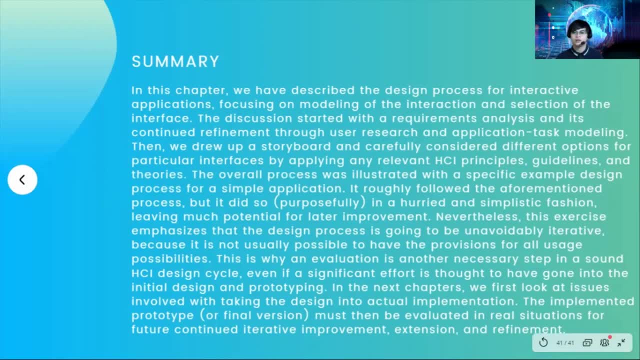 simple application. so it roughly followed the aforementioned process, but it did so purposely in a horrid and simplistic fashion, leaving much potential for later improvement. so, nevertheless, this exercise emphasizes that the design process is going to be unavoidably iterative, because it is not usually possible to have the provisions for all usage possibilities. 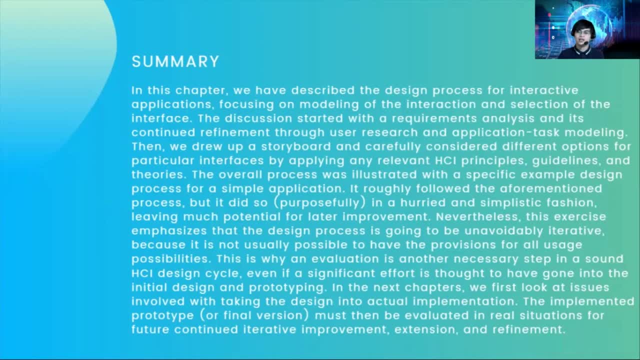 so this is why an evolution is another necessary step in the sound of HCI design cycle, even if a significant effort is thought to have gone into the initial design and prototyping. okay. so in the next chapters we first look at the issues involved with taking the design into actual implementation. so the